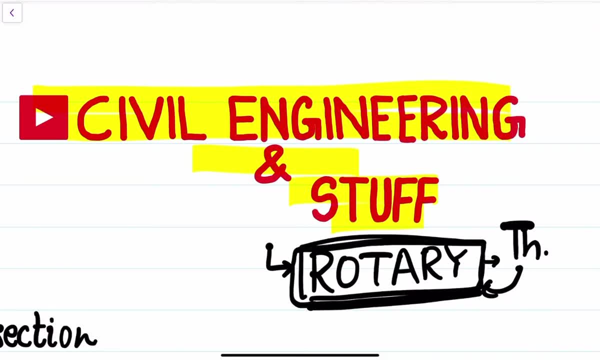 When should we go for Rotary Intersection and what are the design parameters for a Rotary? So that is what we are going to discuss in this video lecture. Mainly, this lecture will be focused on theoretical concepts. We are going to do a small numerical regarding one of the design parameters, But on and all the discussion will be theoretical concepts. 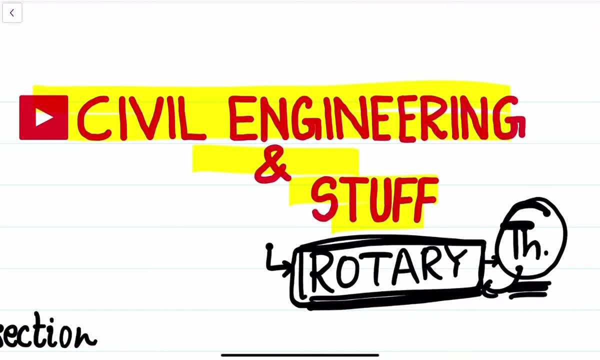 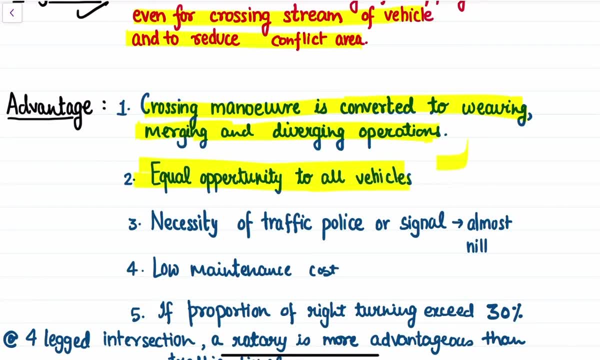 So this is the video And in future, as in when a numerical on Rotary Intersection will be discussed. So this is the video And in future, as in when a numerical on Rotary Intersection will be discussed, to move across the intersection without much compromising with their speed. 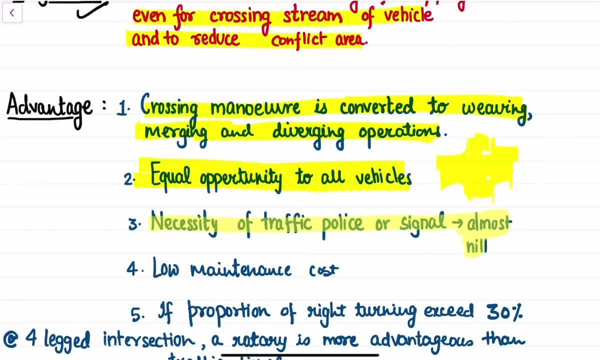 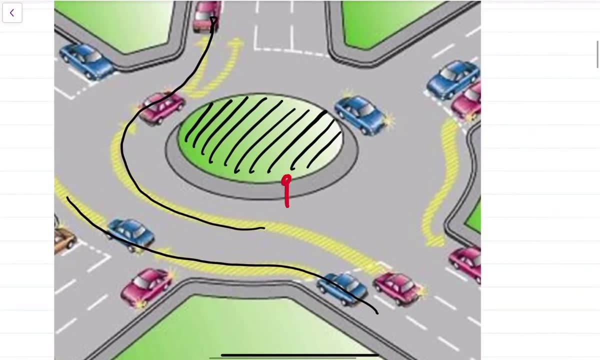 The necessity of traffic police or signals is almost avoided In case the traffic volume is very high, especially in the peak hours, if the traffic volume is very high. so only in that scenario we will install one traffic policeman. or let us say there is too much traffic coming from one direction. 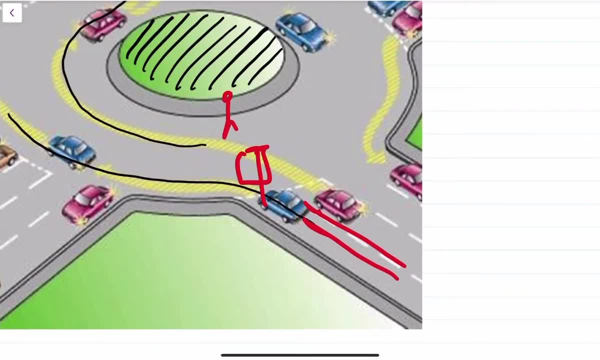 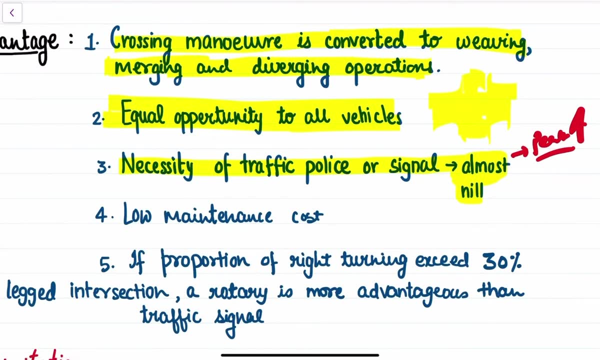 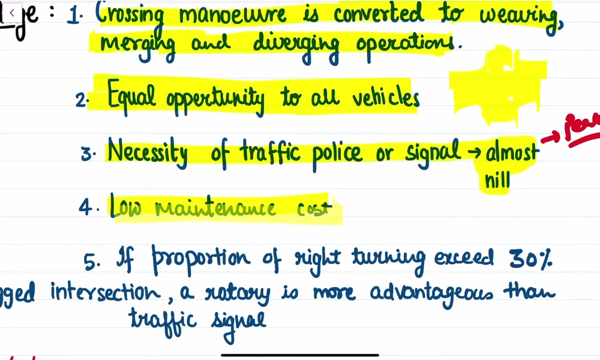 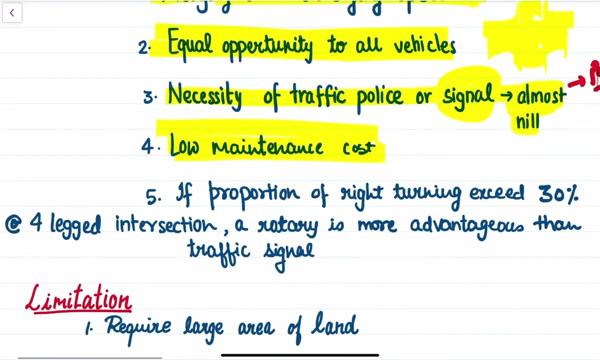 so then only we will install a traffic signal, Otherwise there is no requirement. The traffic stream adjusts itself along the island. There is very little cost of maintenance for a rotary compared to the traffic signals. Another advantage is if the proportion of right turning traffic exceeds 30%. 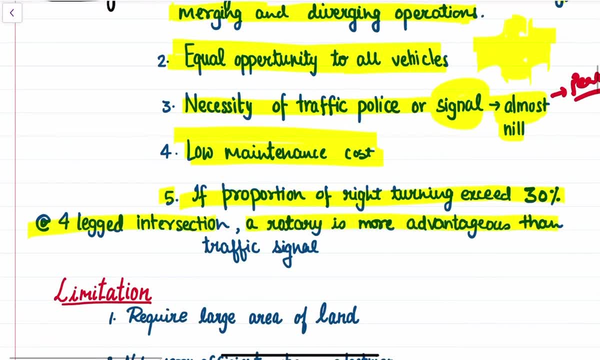 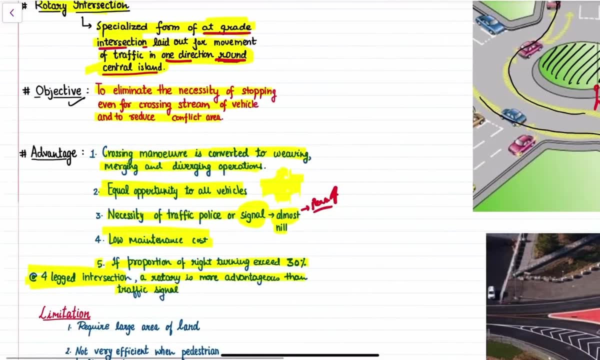 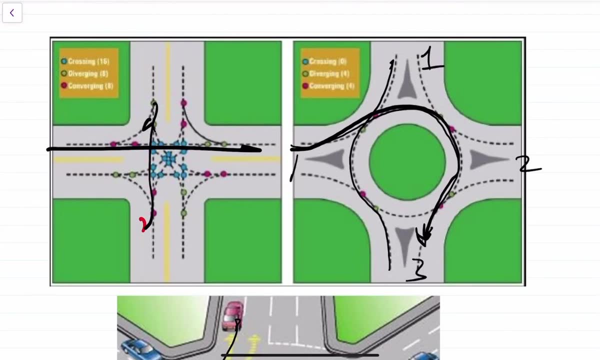 for 4-leg intersection. a rotary is more advantageous than the traffic signal. So by 4-leg intersection we mean these are the legs: This is leg 1,, this is leg 2, leg 3 and leg 4.. 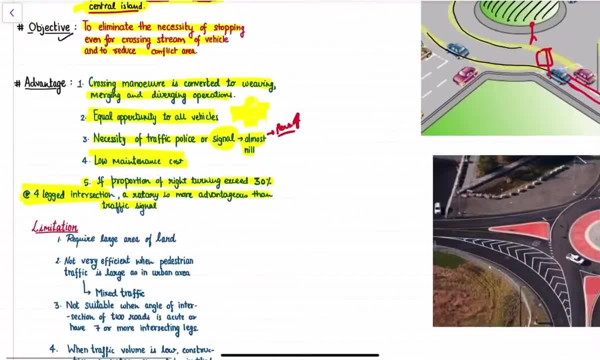 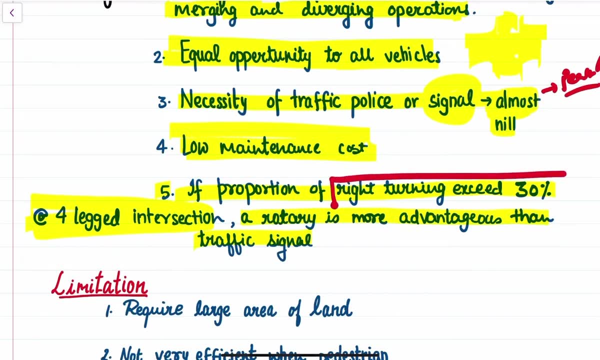 So in case of 4-leg intersection, if the right turning traffic, if the right turning traffic exceeds 30%, then rotary is more advantageous than traffic signal. Because in traffic signals, what do we have? We have traffic coming totally at halt in the red light. 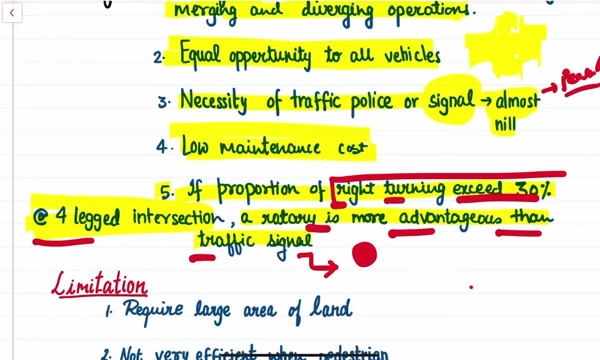 While in rotary that is not the scenario. In rotary the idea is the traffic is constantly in motion. Wherever the vehicle has to go, they are always in motion. So in case where the traffic volume is higher, especially the right turning traffic is higher than 30%. 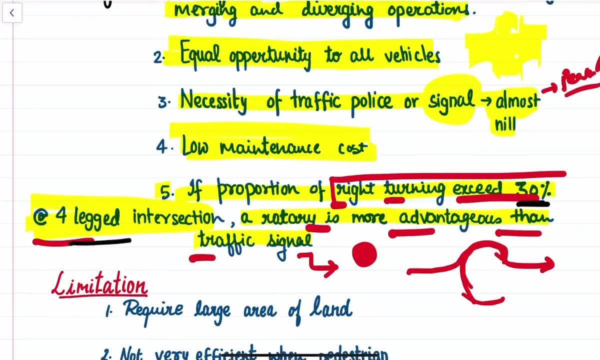 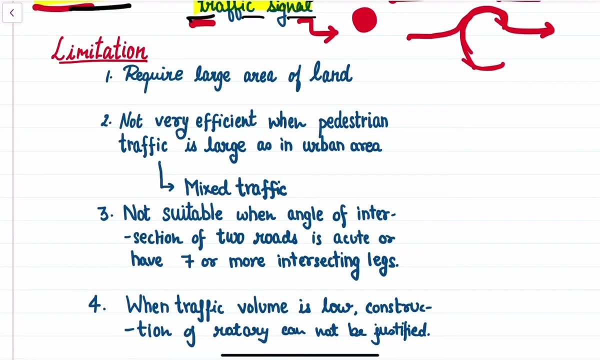 exceeds 30%, then we have to look into the possibility of construction of rotary before we go for the installation of traffic signal. Now there are certain limitations also of rotary. The limitation is that first of all, it requires large area of length. 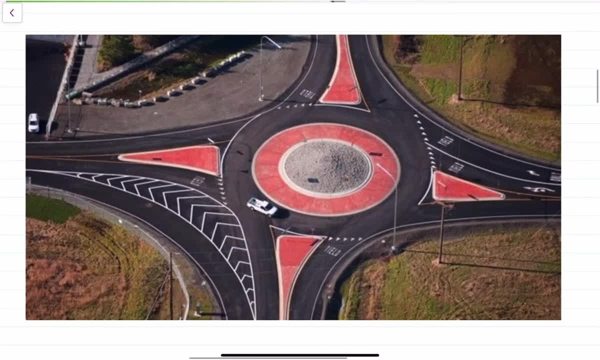 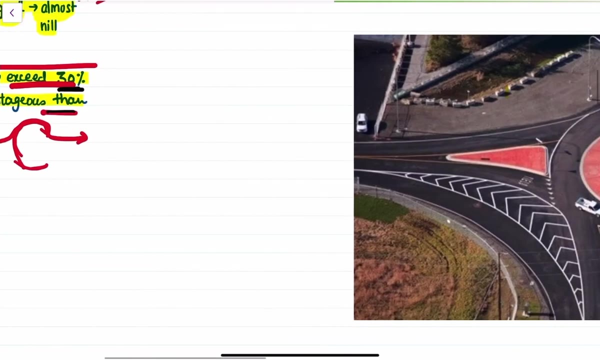 This is a practical or an actual image of a rotary, And you can see how much area is required for the construction of this rotary. So that is one limitation. Suppose we do not have that much area, then of course we have to look into some other traffic management scenario. 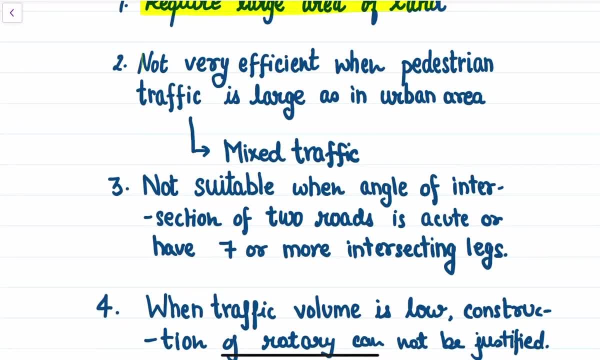 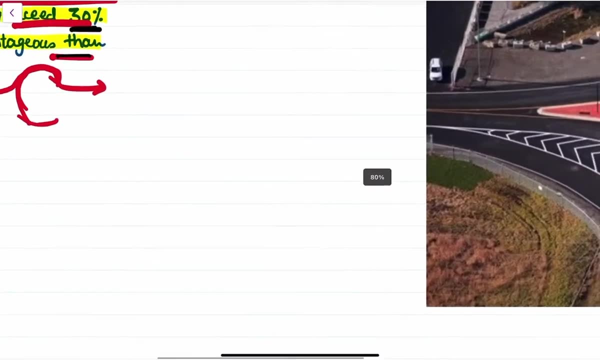 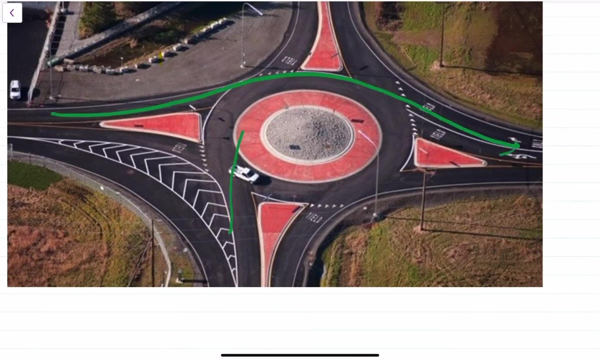 Another limitation is that it is not very effective when pedestrian traffic is large Or the efficiency of rotary is limited in case of mixed traffic, For homogeneous traffic, that is, in case we want to control the movement of vehicles across the rotary intersection. That is the scenario. 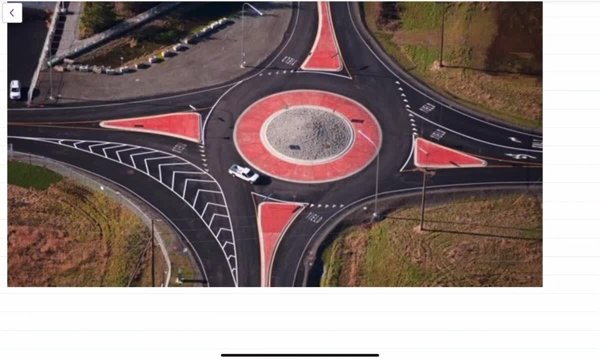 If that is the scenario, then the functionality of the rotary is fairly high, But in case we want to have pedestrian crossing also, like we have just now discussed, that the idea is that the traffic should always be in motion, The vehicles should never stop. 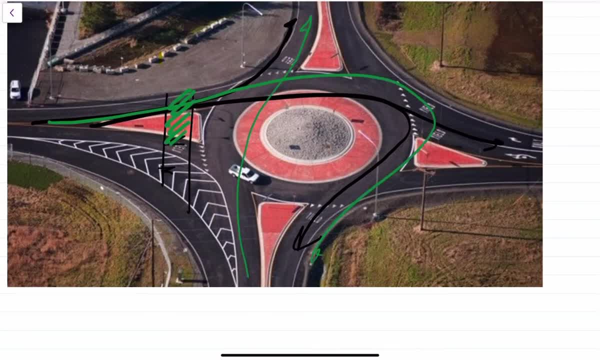 They should be always in motion. So having pedestrian crossing, there may be a location where the rotary is in vicinity of population. So in that case if we have to construct zebra crossing, then the whole idea of constant movement of traffic is minimized. 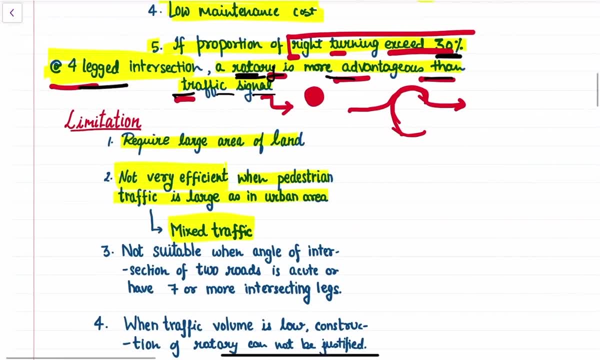 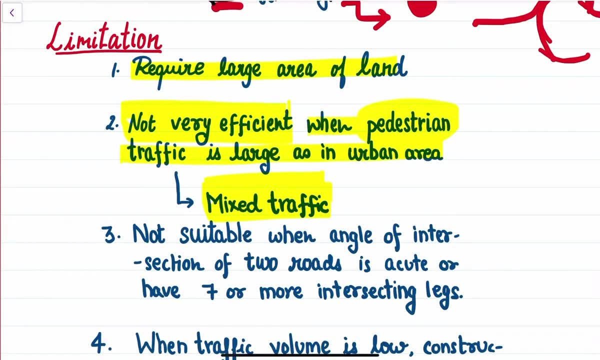 We have to look into the safety of pedestrians also. So that is a limitation of rotary, that in case of mixed traffic conditions, in case of like, if you have cycle like, cycle is also moving on the rotary side. we have pedestrians also moving on the rotary side. 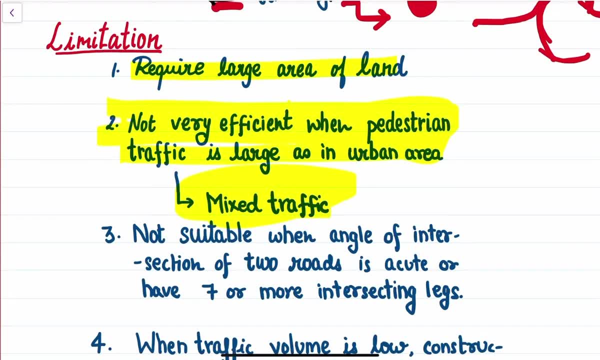 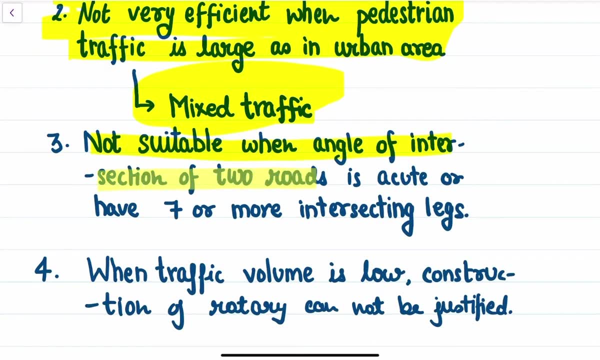 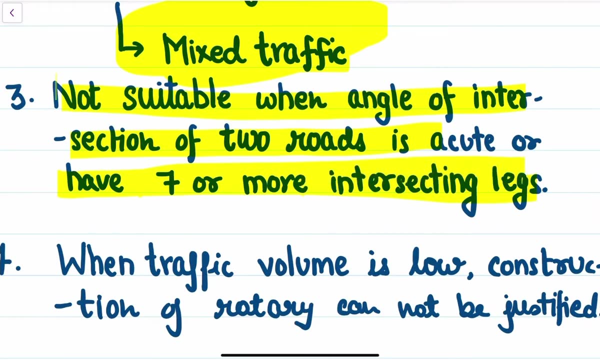 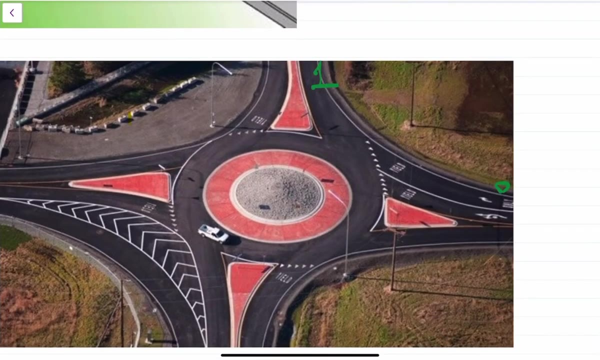 So in case of mixed traffic scenario, the efficiency of rotary is minimized. Construction of rotary is not suitable when angle of intersection of two roads is acute or have seven or more intersections or intersecting legs. So we are seeing that, like conventionally, rotary is having four legs. 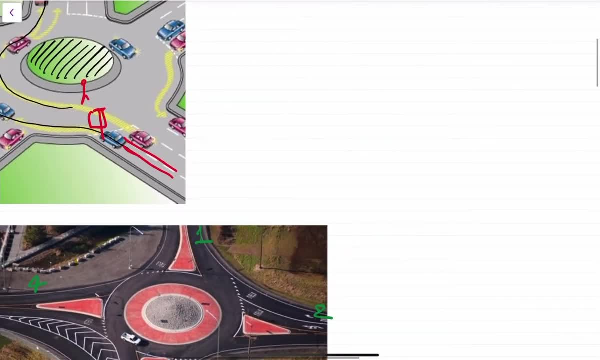 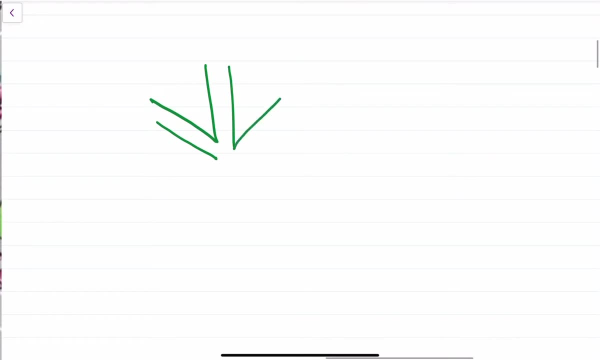 And even in these four legs, suppose the overall or the natural intersection is like this, The intersection is like this. So in that case of the construction of rotary like becomes a very critical design parameter, right Where the angle is very acute, right. 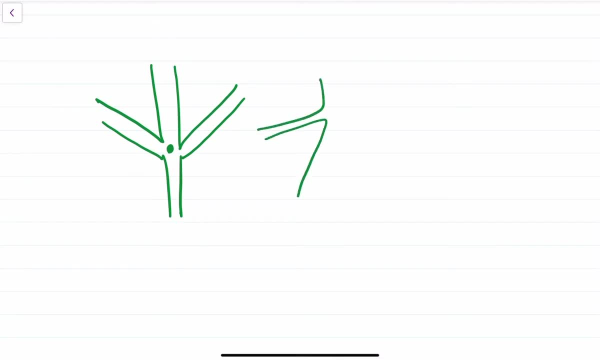 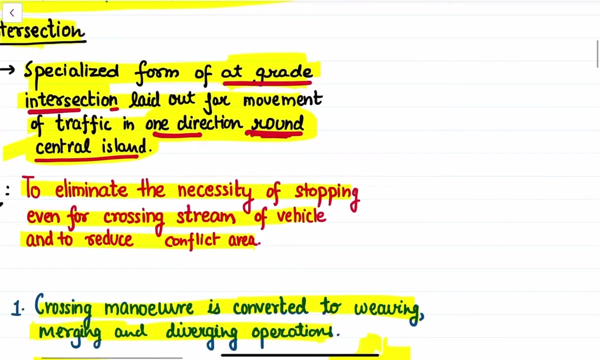 Or in case we have multiple legs intersecting. So again there, construction of rotary is not a desirable scenario, right, Though it can be constructed and it can work efficiently. But it causes certain amount of confusion and everything. So that is why it acts as a certain limitation of rotary, right? 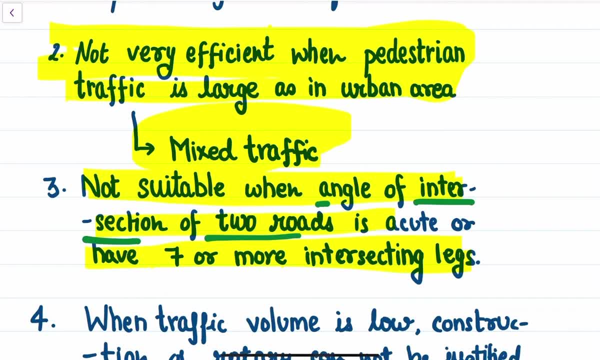 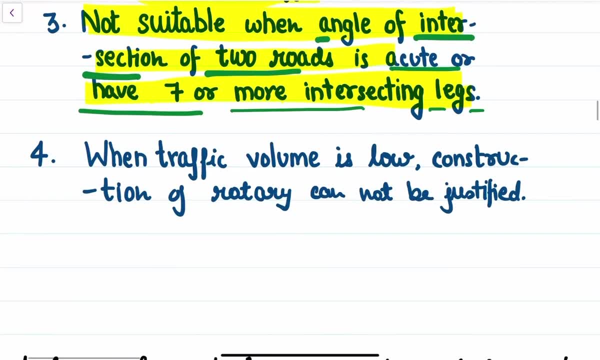 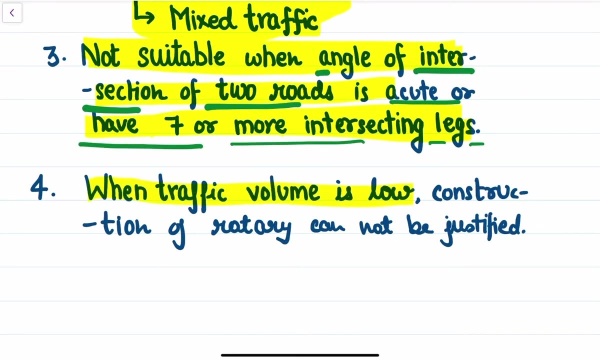 When the angle of intersection of two roads is acute or have seven or more intersecting legs, then the efficiency of rotary decreases. Another limitation is that we cannot construct rotary when traffic volume is low right Because construction of rotary, initial cost of construction of rotary, is very high right. 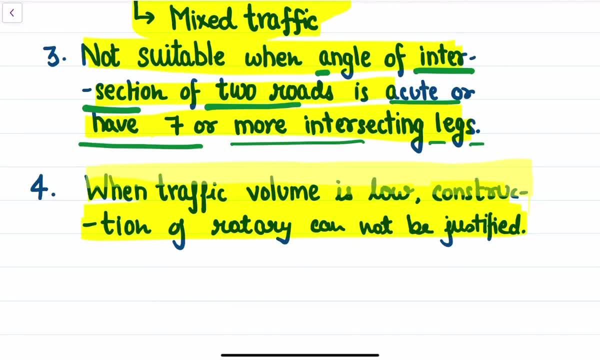 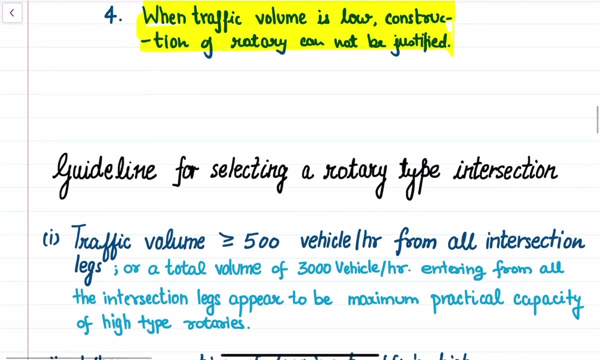 Compared to the installation of traffic signal. So in case the traffic volume is low, then the installation of or the construction of rotary in that intersection is not advisable. So there are certain guidelines for construction of rotary type intersection. The first is: when should we go for? 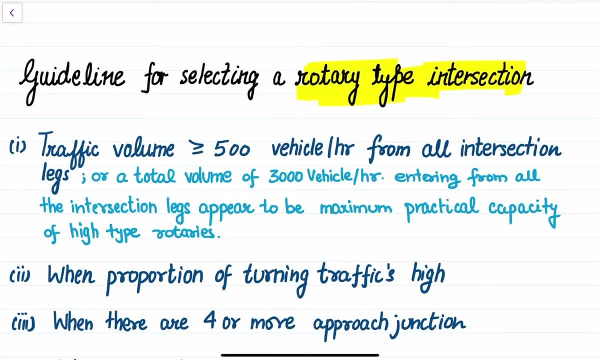 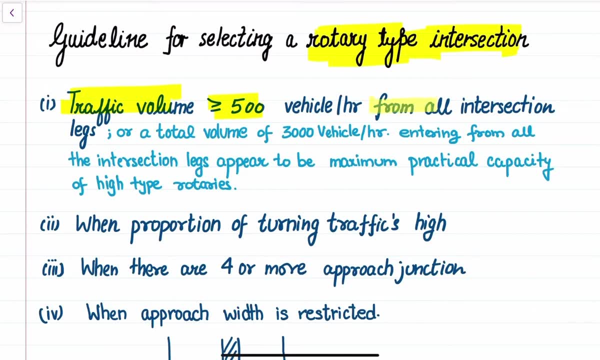 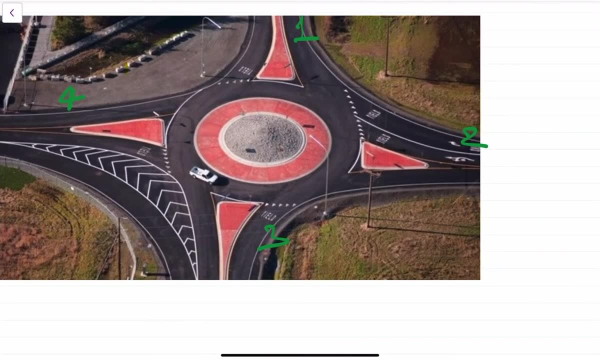 The construction of rotary along an intersection. So the first one is that, in case the traffic volume is greater than 500 vehicles per hour, for all intersection legs, This means, this means that in each of the legs, in each of the legs, 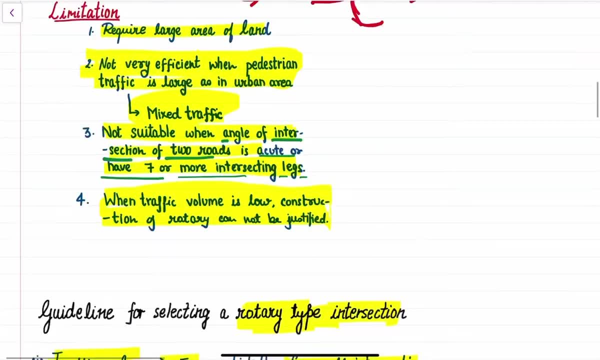 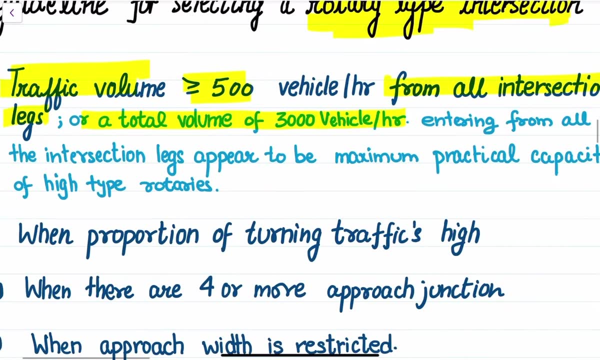 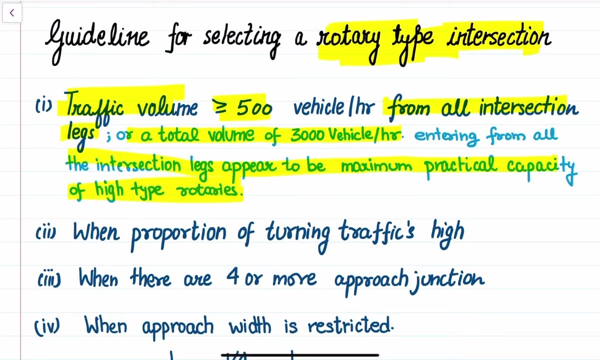 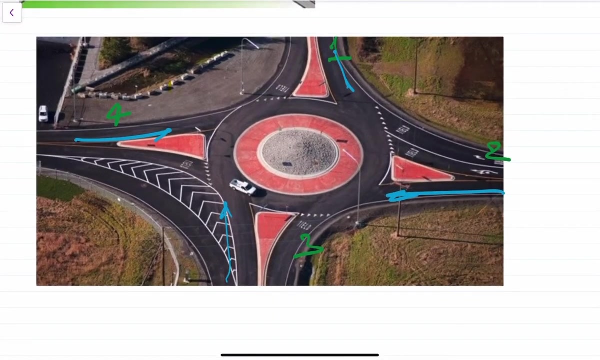 we have a traffic volume of 500 vehicles per hour, or a total traffic volume, or a total traffic volume of 3000 vehicles per hour entering from all the intersecting legs appear to be maximum practical capacity of high tide rotary. This means either 500 vehicles per hour from each leg or throughout the intersection. 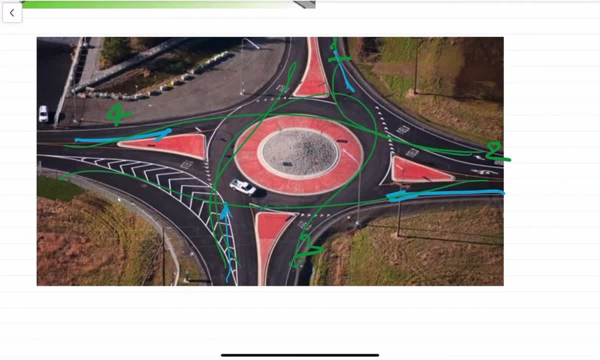 Throughout this intersection we have a traffic volume movement of 3000 or 3000 plus vehicles per hour. So if that is the like, the higher traffic volume is moving along the intersection. So then only we should look into the possibility of construction of rotary in that intersection. 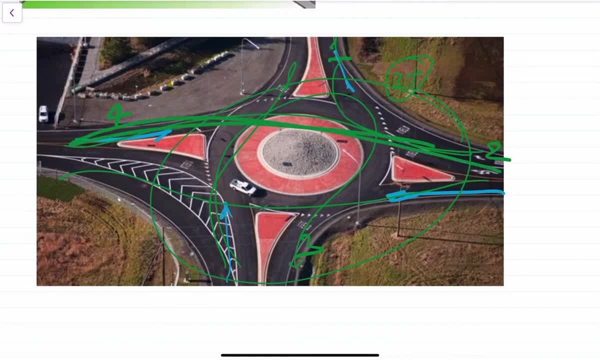 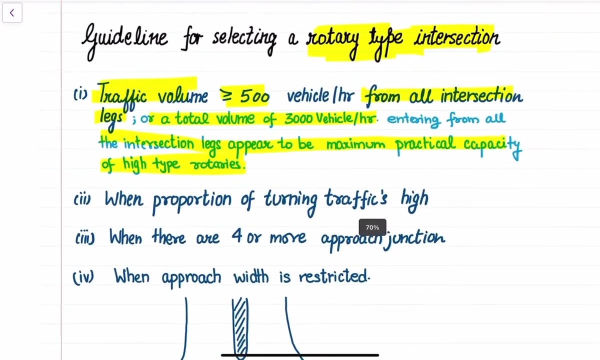 Because, since traffic volume is high, we want the constant movement of traffic along this rotary intersection. All right. So that is one of the primary guidelines that is needed to be taken care of When we we have to look if we are going to construct for a rotary in that intersection. 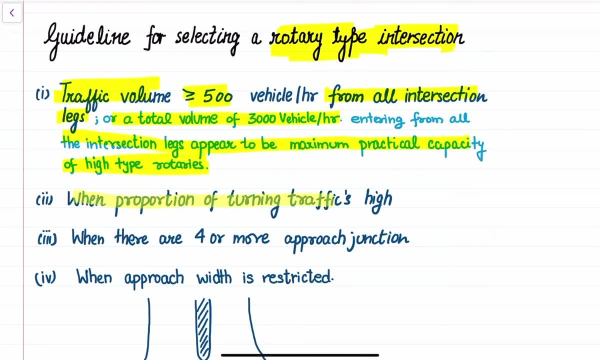 In case an intersection is having higher amount of right turning traffic, In case when proportion of turning traffic is high, or if we say, like right turning traffic, If right turning traffic is high, then we go for rotary construction. In case there are four or more approach junction, then again we go for rotary intersection. 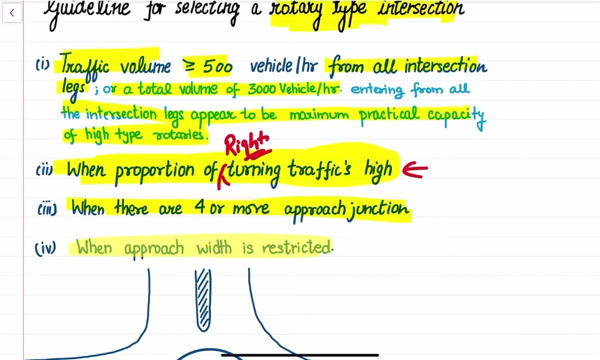 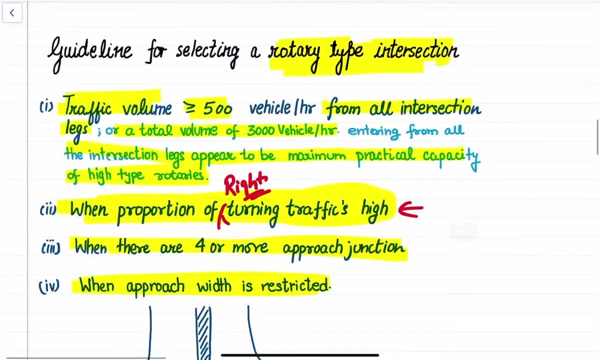 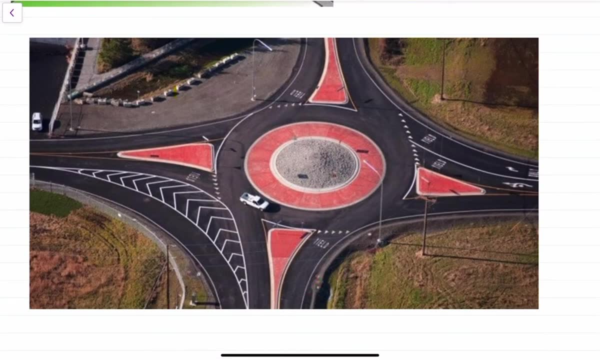 And when we have the approach with restricted right, In that case we go for the construction of rotary type intersection. All right, So just to be just for reminder, this is a rotary. So if you observe, if you observe, we have one phantom. 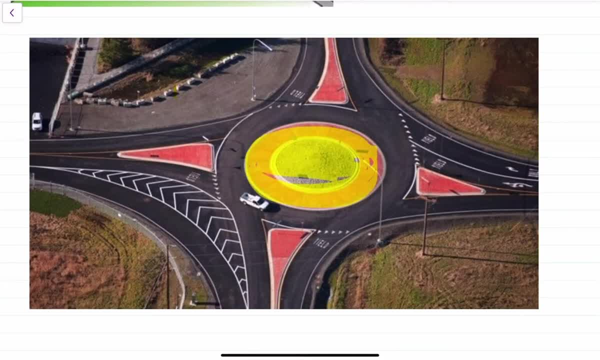 One central island right. We have certain restrictions around the rotary. We have we have legs 1,, 2,, 3, 4.. In this case we have four legs right. We have certain curve path. We have certain width available. right. 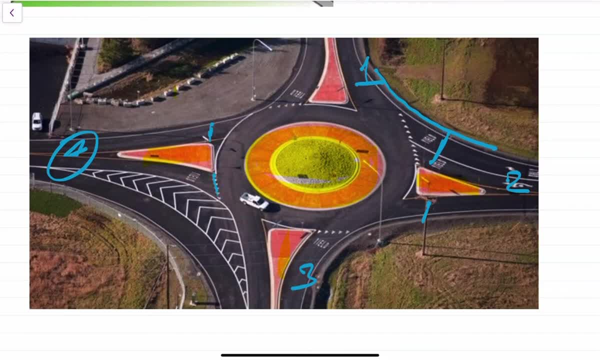 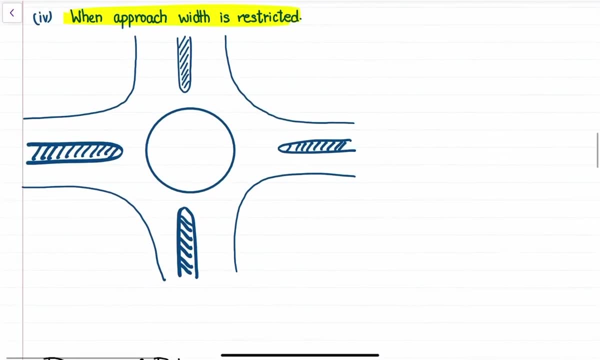 We have certain width available that varies. So we are going to discuss what all these parameters are called in a rotary. So let us discuss through a diagram. So let us say: this is our rotary. All right, This is our rotary. 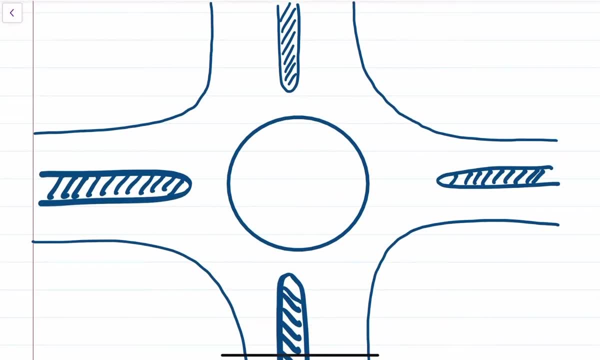 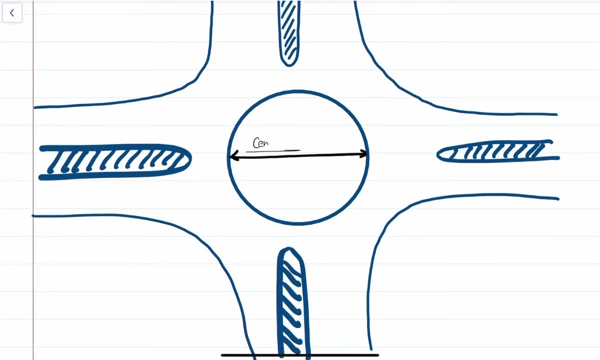 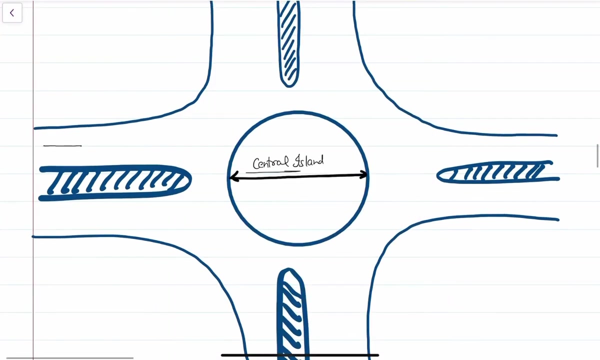 Now, in this, in this, this central island, this is the, this is the central island, Central island, And this whole diameter is called as central squared diameter If a vehicle is approaching, if a vehicle is approaching through this direction. 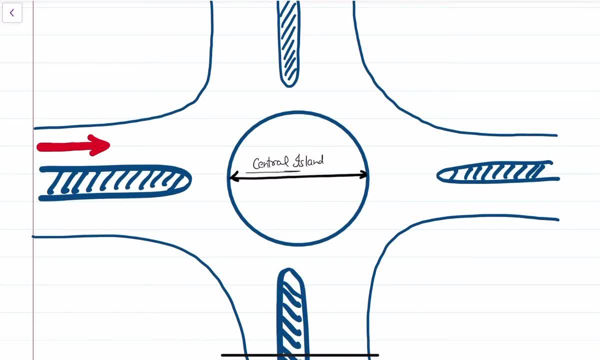 So there is certain width available. there is certain width available for this vehicle. So this width is what we call as the. this width is what we call as the entry width. This width is what we call as the entry width And of course, the vehicle will move through, the entry width will weave out and if let 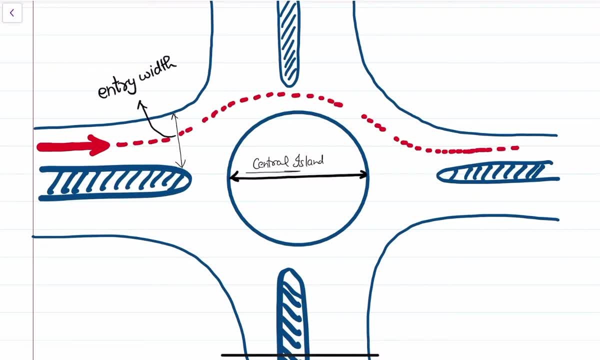 us say he wants to go in this leg and will go here, right, So this width available, this width available is what we call as the entry width, is what we call as the exit width. right, This is what we call as the exit width. This 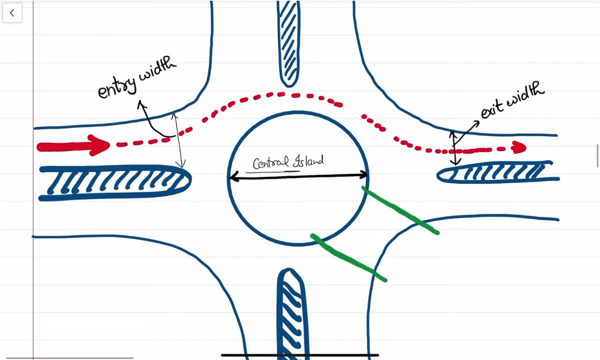 section. this section of row tree. this section of row tree is called as the weaving length and this is called as the. this is called as the weaving width, this is called as the weaving width right. So, in each direction, this is: this is the weaving length, this. 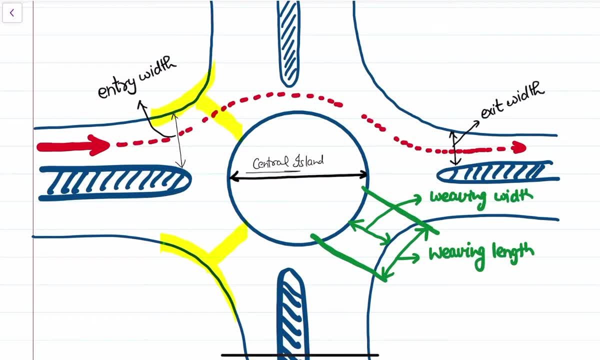 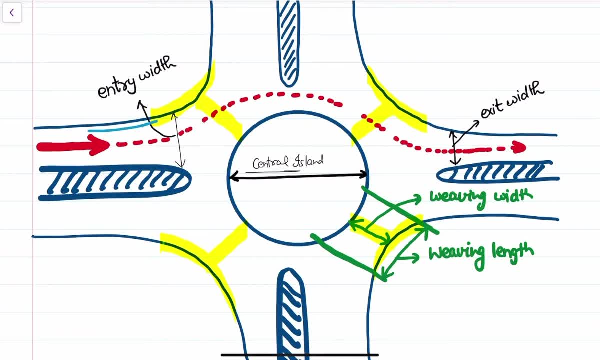 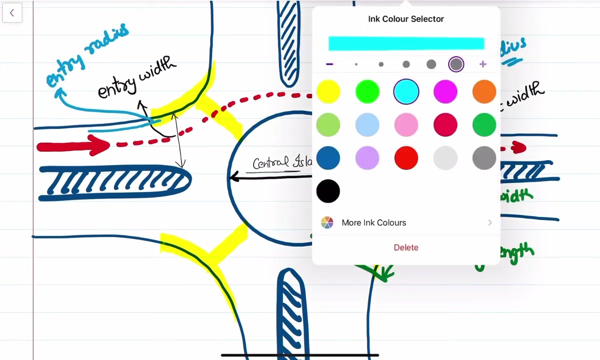 Right from where the curvature starts. right from where the curvature starts is what we call as the entry radius, And this will be called as the exit radius, And this is called as the exit radius. Now, in this rotary section, in this rotary section, we have this central island, this is the, this is 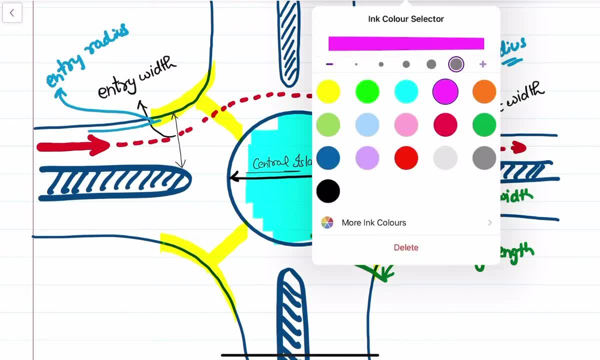 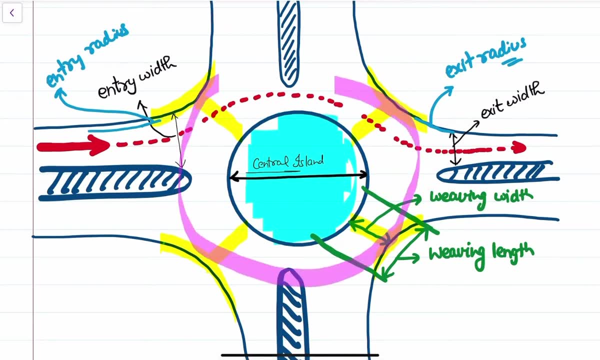 the central island. along with that, if you observe, there, there is another circle that is inscribed right. this is the another circle that is inscribed. so the diameter of this right from here to here, the diameter from here to here, is what we call as the inscribed circle. diameter inscribed circle. 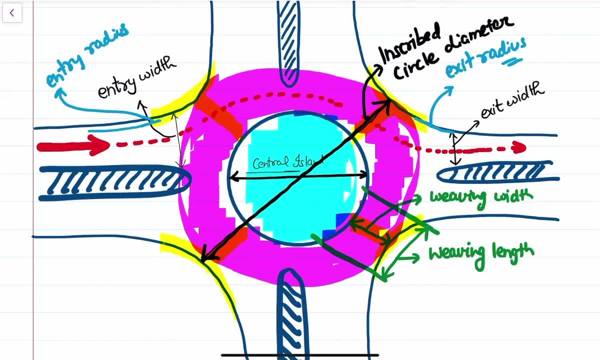 diameter, and this width between the inscribed circle diameter and the central outer of the central island is what we call as the circulatory carriageway width. this is what we call as the circulatory carriageway width. this is what we call as the circulatory carriage way. this all right. 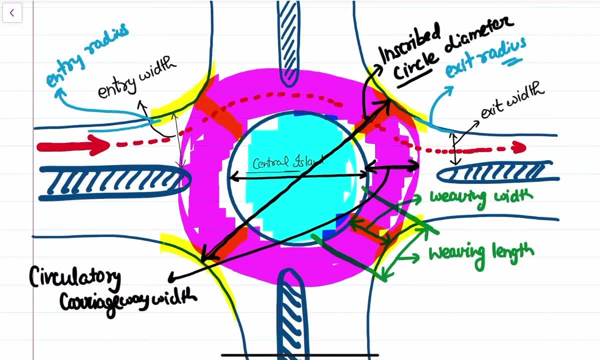 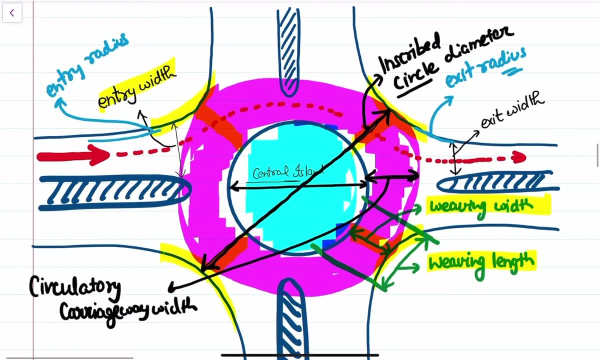 so important parameter in for you to remember here, important parameters are these, leaving with living length, the entry width, the exit, exit width, entry radius or exit radius, the radius of central island. these are the mean parameters. apart from that, we have these what we call as the inscribed circle diameter and the circulatory carriageway width. alright, 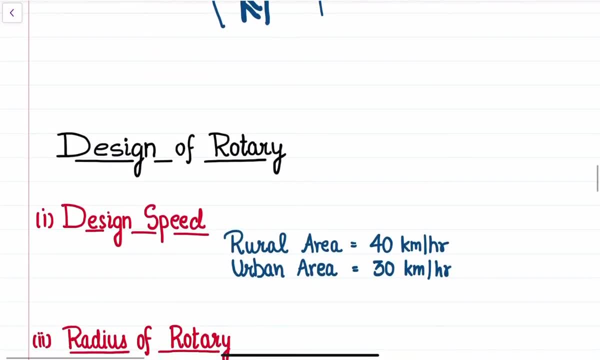 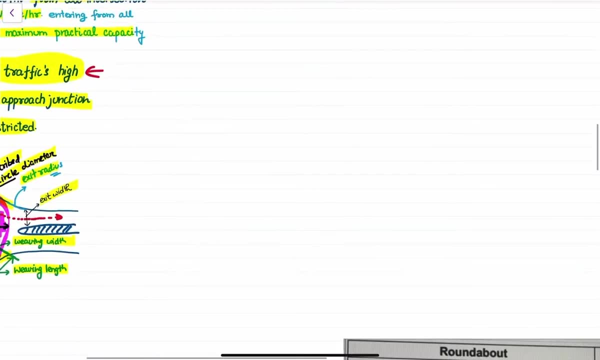 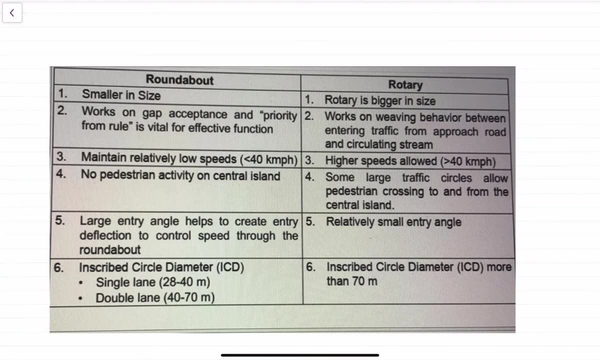 So next we have is the design of rotary. So before I move to the design of rotary, let me first of all discuss the difference between rotary and roundabout. Let me discuss the difference between rotary and roundabout. So one and all, the structure of rotary and 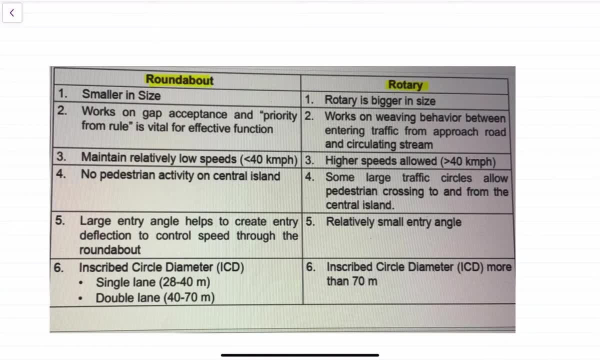 roundabout is same. right structure wise is same, but your roundabout is smaller in size compared to that of a rotary. Your roundabout is smaller in size compared to that of a rotary. Second is that your roundabout works upon the gap, acceptance and priority rule. Your 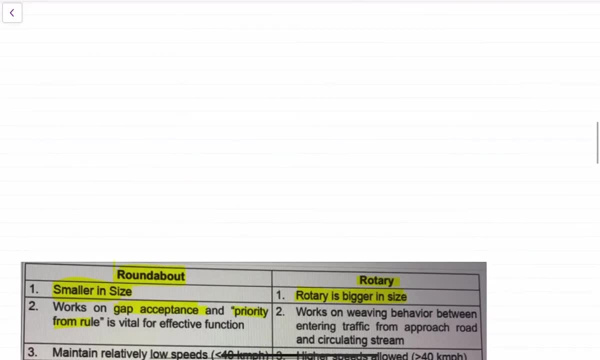 roundabout, being smaller in size. So what happens is I will just draw, for example, if this is your roundabout, For example, this is your roundabout, If this is your roundabout, If this is your roundabout and this is your row tree. 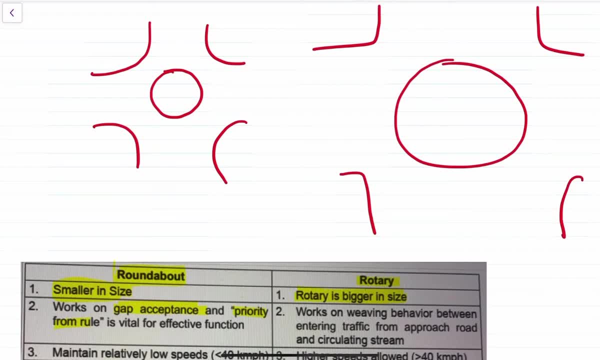 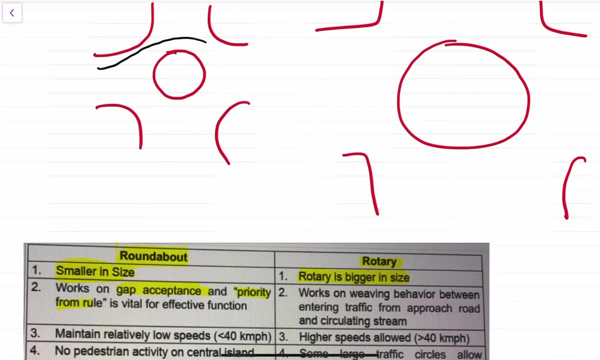 This is your row tree, Okay, So roundabout being smaller in size. so there is not much width available, Especially, not much viewing width is available. So what happens is that there are movement of vehicles in every direction. Right At the same time, there will be movement of vehicles in every direction. 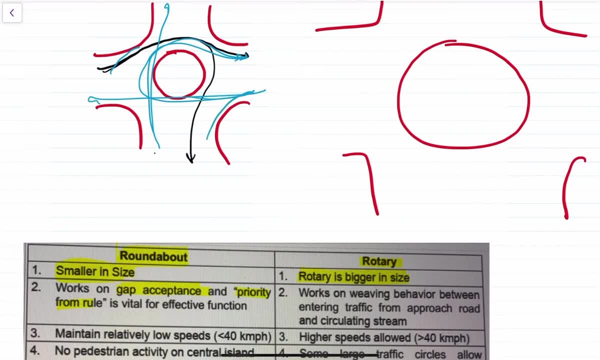 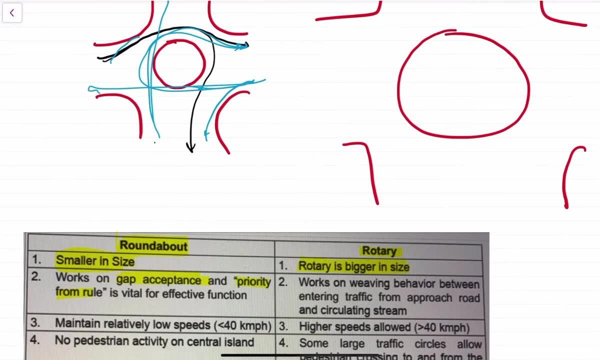 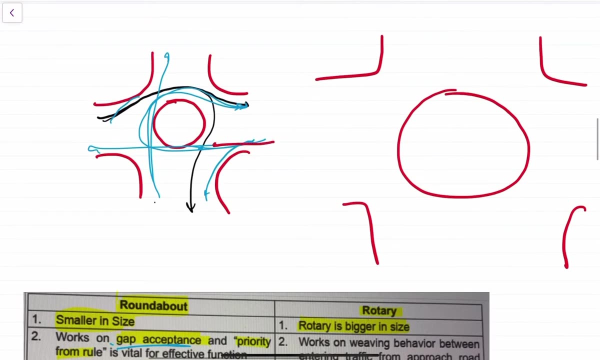 Right, There will be movement of vehicles in every direction. So what happens is this roundabout works upon the gap acceptance criteria. This means that if a vehicle is approaching from here, and there is any vehicle that is approaching from this direction, so one will slow down and the other will pass. 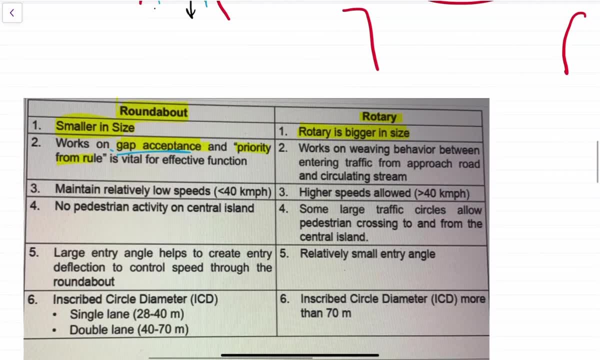 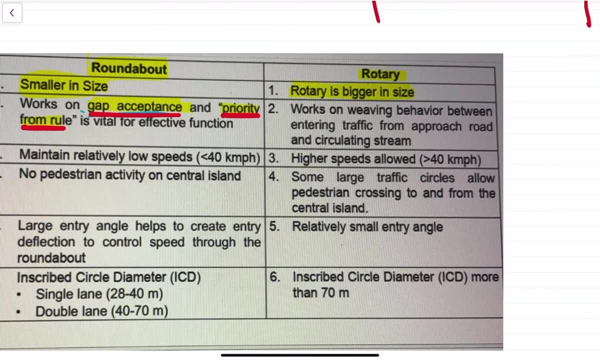 Right, One will slow down and other will pass Right. So it works upon the gap acceptance. So it works upon the gap acceptance criteria or the priority rule, While in row tree the movement is based upon the viewing section, Based upon the viewing behavior. 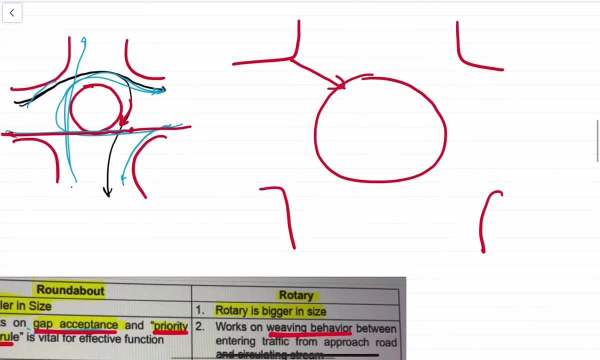 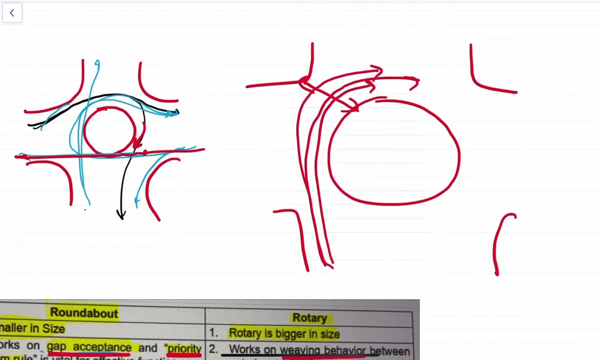 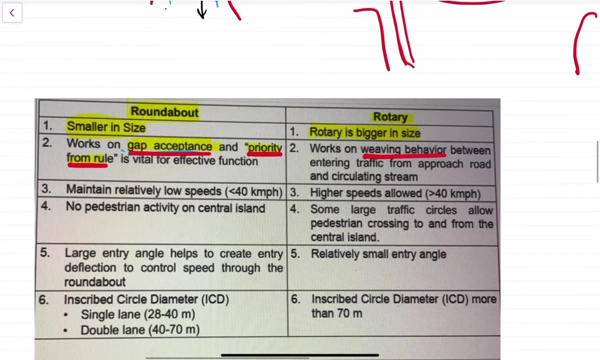 This means here there is ample amount of viewing width available. So in case like if there is multiple vehicles moving in the same direction, so they have certain, like ample amount of space available to move from one place to another, Right, So it works upon the viewing behavior. 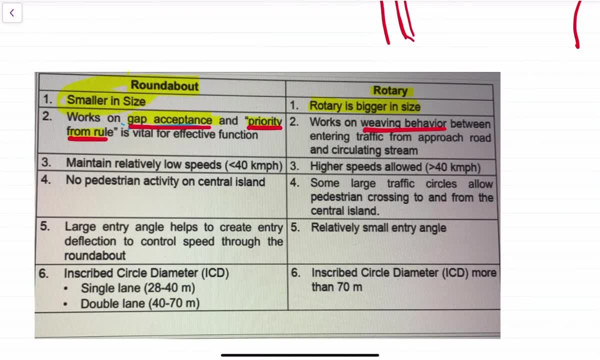 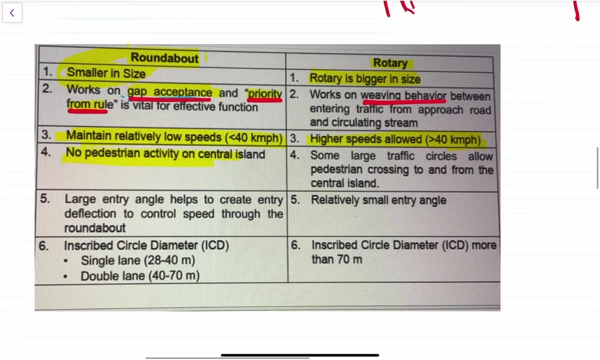 So this is the roundabout. The speed is maintained So in case, like in the roundabout being smaller, So relatively low speed is maintained in your roundabout, while in row tree relatively higher speed is maintained In roundabout. no pedestrian activity is there in the central island. 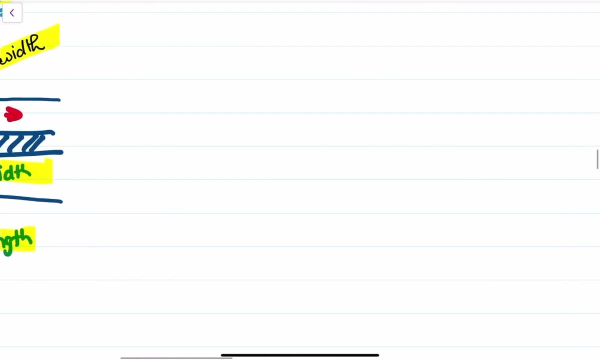 So central island- we have discussed What is central island, The central part, Right, This is your central island. So if we talk about this, This is your central island. So, in roundabout, central island being small, 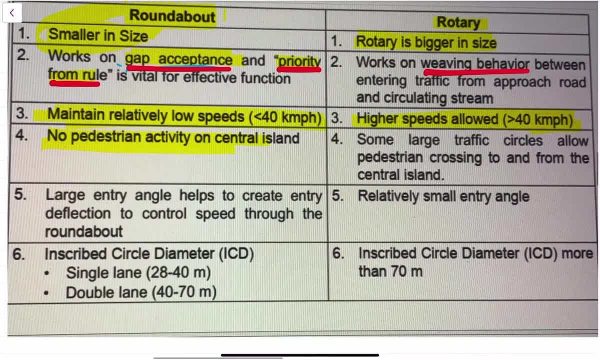 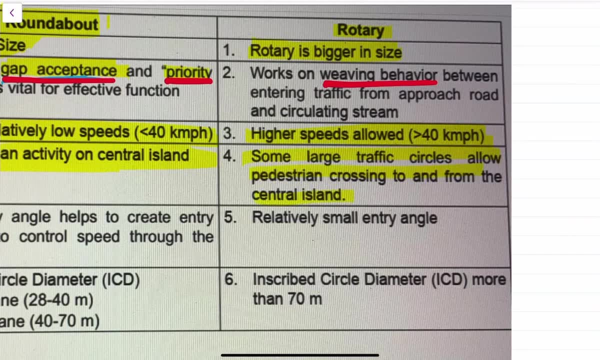 smaller so there is not much activity can be planned in the in the central island, while rotary have a bigger central island. so it can be used either as a pedestrian crossing. it can be used either as a small park. it can be used for multiple purposes. right, your roundabout has. 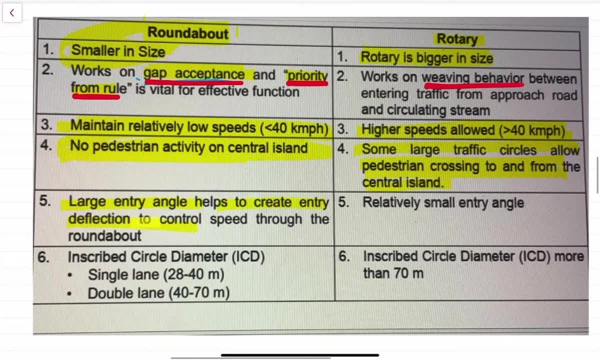 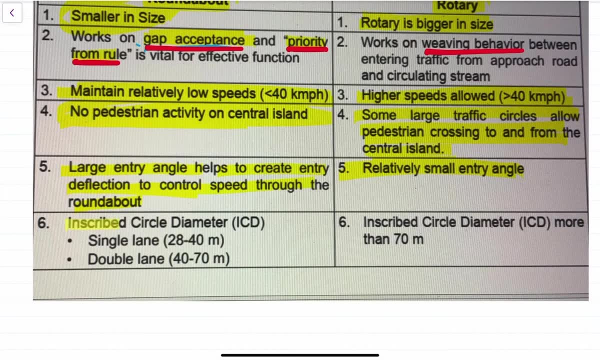 large entry angle that has to create entry deflection and to control speed through the roundabout, while the entry angle is relatively smaller in the rotary, the inscribed circle circle diameter for a roundabout is 28 to 40 meter for a single lane, 40 to 70 meter for a double lane. 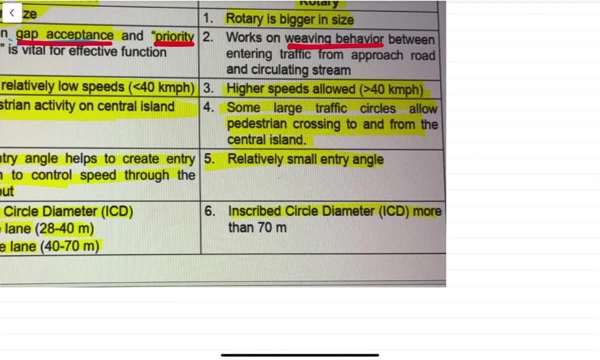 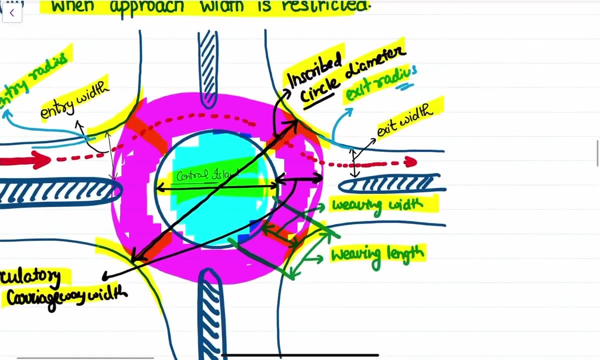 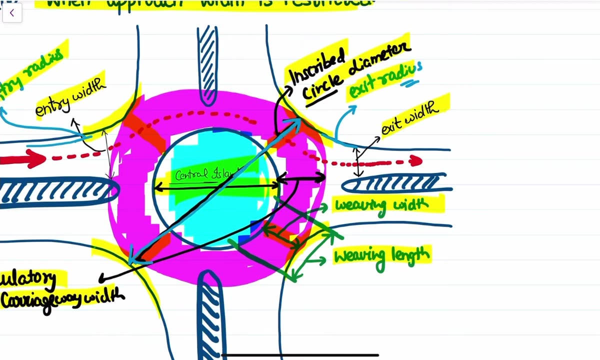 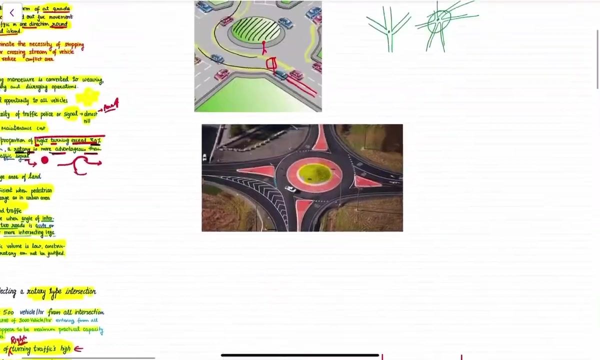 while the inscribed circle diameter for rotary is 70 meters. inscribed circle diameter. what is inscribed circle diameter? this one, the diagram, is now become hotspot, but this is your inscribed circle diameter. this is your inscribed circle diameter. okay, if we look into this image here, this is: this is our inscribed circle diameter. 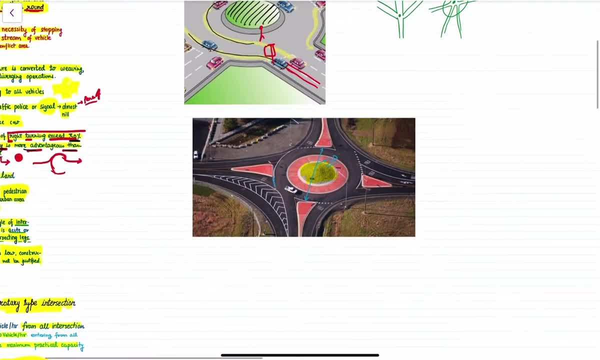 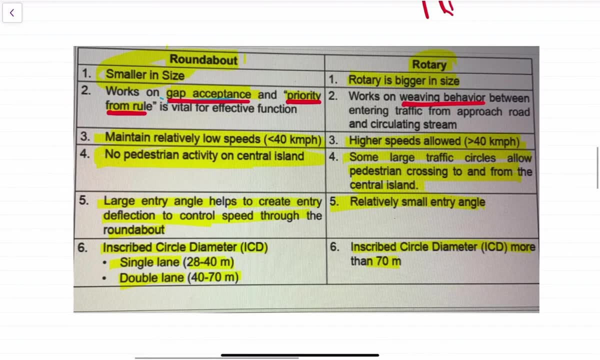 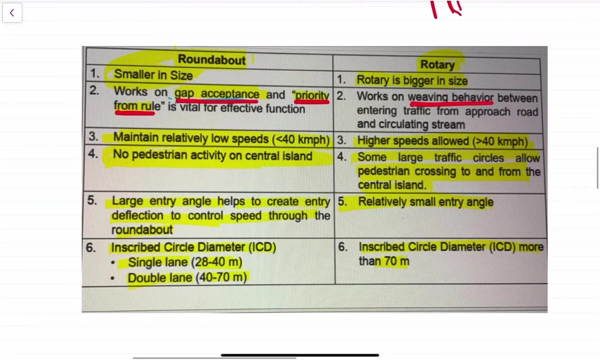 inscribed circle diameter. this is our icb clear. i hope it's clear to you all right, so this is the basic difference between uh, rotary and roundabout. these are the basic difference between uh, rotary and roundabout. construction wise- same, but dimension wise. and uh, like there are certain. 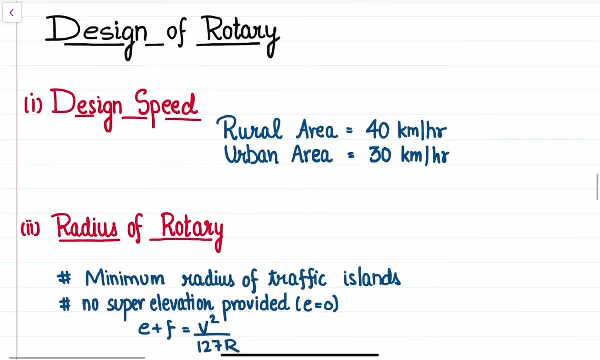 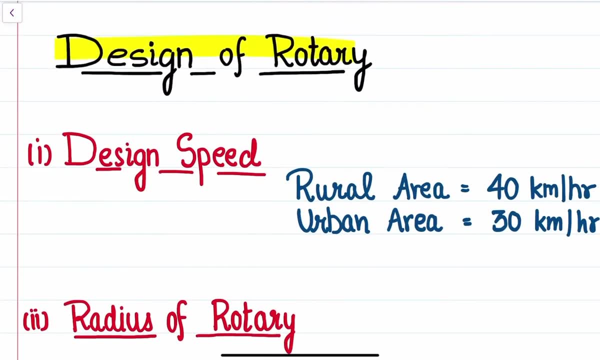 other parameters on which these they differ. right, so it is not an interchangeable term. all right, so now let us discuss about the design of rotary. okay, let us discuss about the design of rotary. so, after deciding the shape of rotary that we are going to, uh, be using- we, there are certain design. 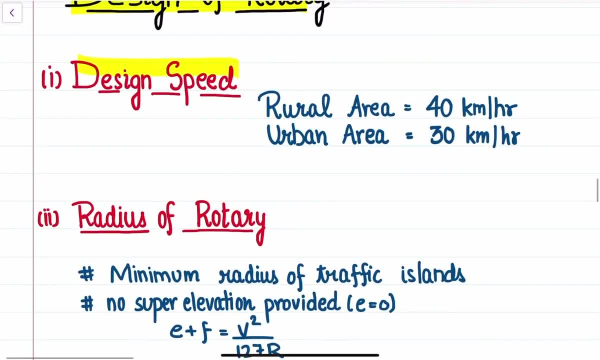 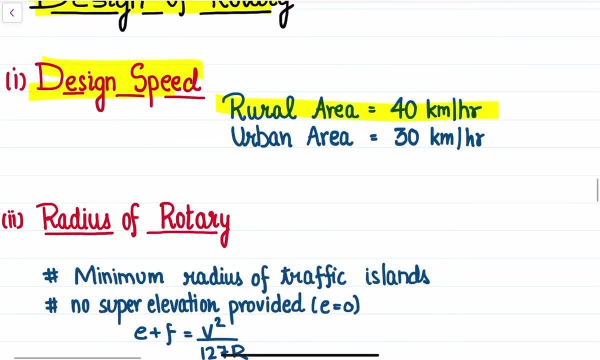 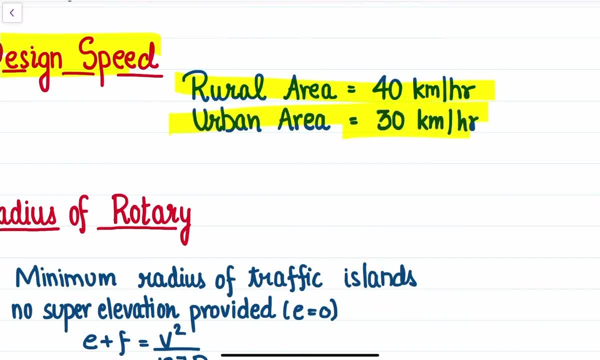 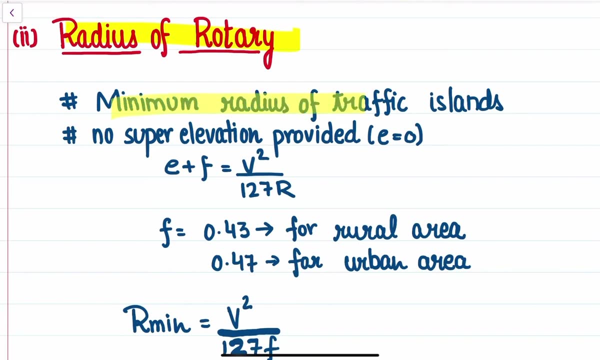 taken, while for urban area speed of 30 kilometer per hour is taken. reason: urban urban area has a higher traffic volume compared to this or area, so like higher speed is taken for the ruler area. then we have radius of rotary and the minimum radius of traffic: island. uh, is what the minimum? 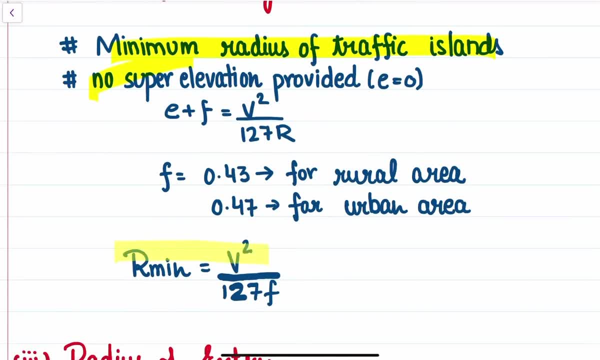 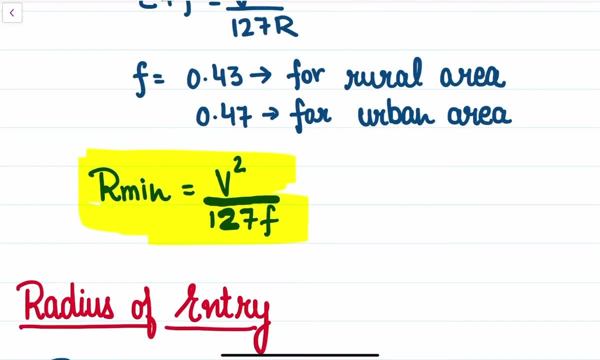 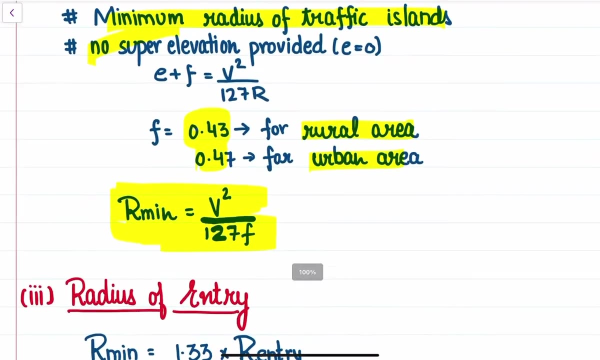 we do not provide any super elevation, and r equals to v square by 127. f is the formula that is used to find out the minimum radius, where f is the coefficient of friction, taken as 0.43 for rural area, 0.47 for urban area. This is the formula to find out the minimum radius. 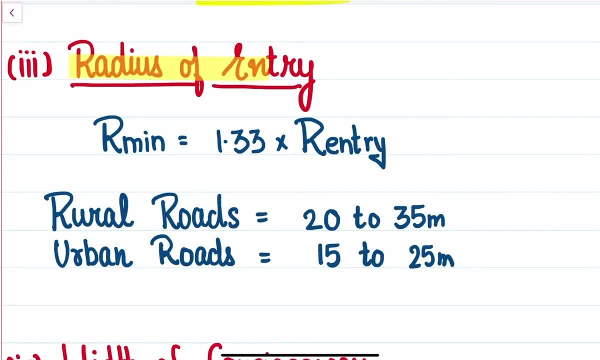 The radius of entry is taken as 1.33.. The minimum radius for entry is taken as 1.33 into r entry, which is for rural road, taken as 20 to 35 meters, and for urban roads, taken as 15 to 25 meters. 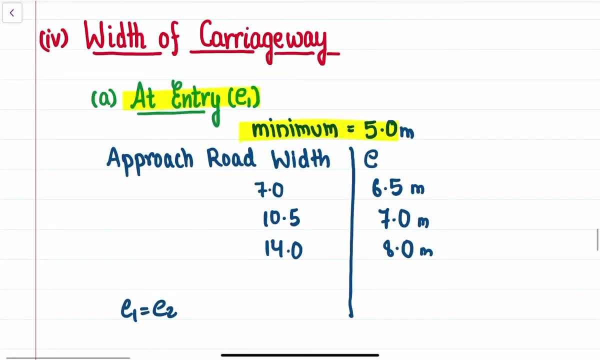 Width of carriageway At entry. the minimum width of carriageway is taken as 5 meters and, depending upon the width of approach road, this width of entry is adopted. So if the approach road width is 7 meters, entry width of 6.5 meters is given. Likewise, 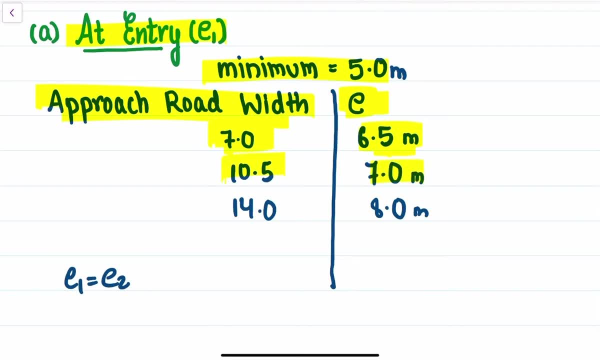 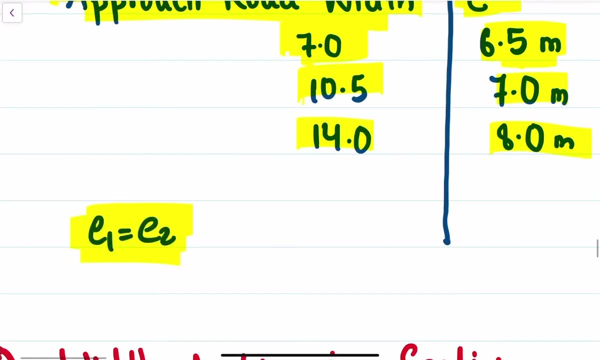 for if the width of approach road is 10.5, then 7 meters is taken. For 14 meter, 8 meter entry width is taken and entry width should be equal to the exit width. It makes sense because the same amount of traffic volume will be going, might be going from that other leg of the road. So 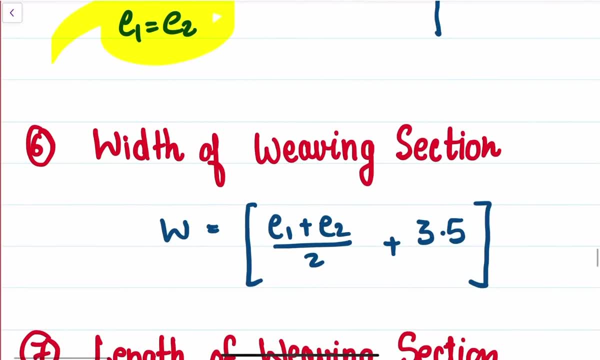 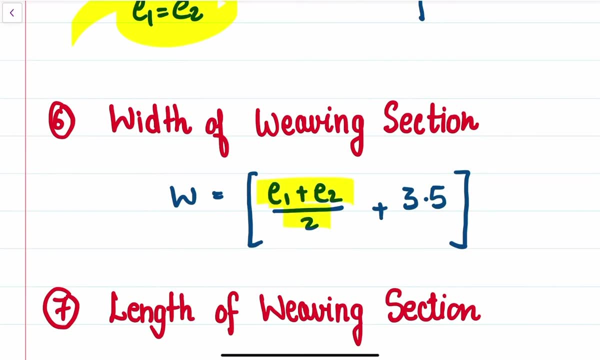 attempt is being made that E1 should be equal to E2.. Width of approach road, Width of weaving section will be equal to E1 plus E2 by 2.. That is entry width and exit width, sum of entry width and exit width divided by 2 plus 3.5.. So that will be the width of. 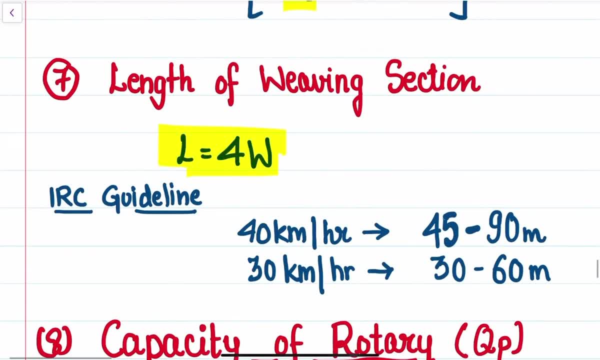 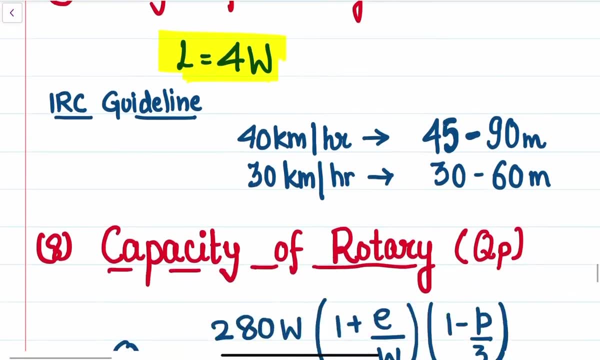 weaving section. Length of weaving section will be 4 times the width of weaving section. Length will be 4 times the width of weaving section And, as per IIC guideline, if you are taking design speed of 40 kilometers per hour, the length should be 45 to 90 meters and for 30 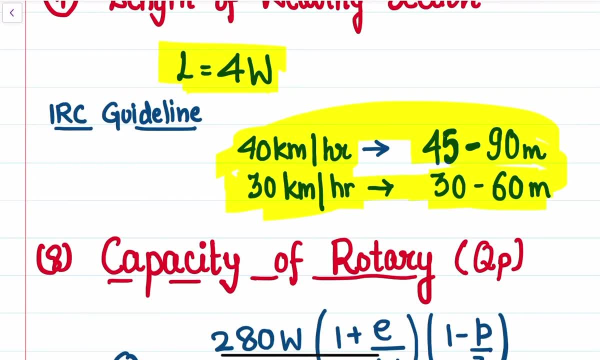 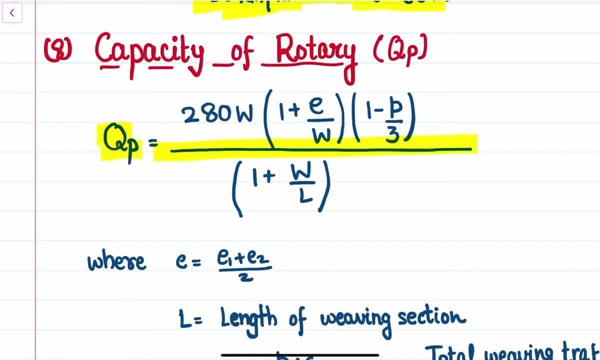 kilometers per hour, the length should be 45 to 90 meters And for 30 kilometers per hour 30 to 60 meters. That is the range that is given by IRC. Now the capacity of rotary is found using the formula: QP equal to 280 W, 1 plus E by W. 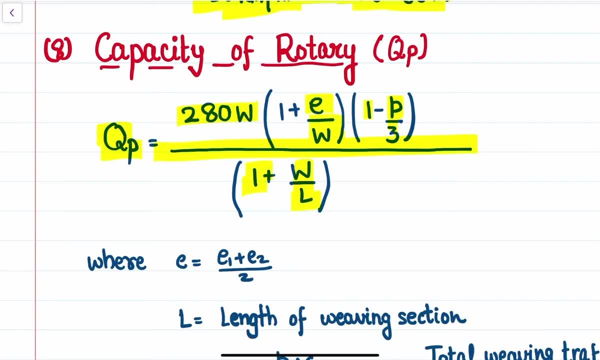 then 1 minus 3 by 3 divided by 1 plus W by L. W is the width of weaving section. L is the length of weaving section. E is the average of the entry and exit width, E1 plus E2 by 2, divided by width of. 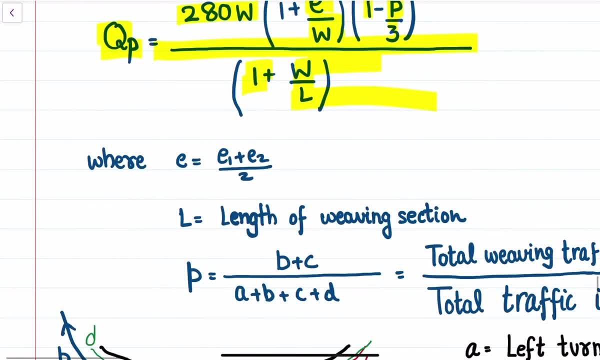 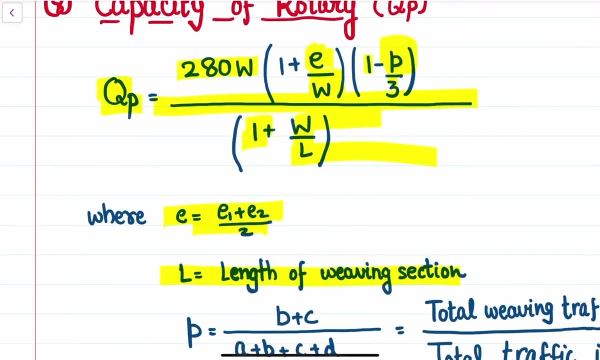 weaving section 1 minus P by 3.. E is equal to E1 plus E2 by 2. L is the length of weaving section P. this is a new term. This is the new term that we are discussing. P is what we call as the weaving. 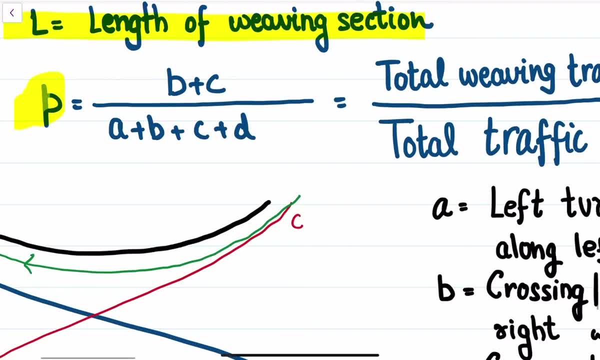 ratio. P is what we call as the weaving ratio, which is equal to D plus C, divided by A plus D plus C plus D. We will discuss about these terms. So P is the, P is what we call as the, what we call as the. 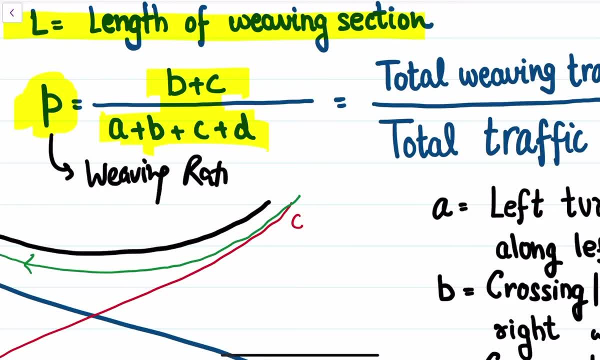 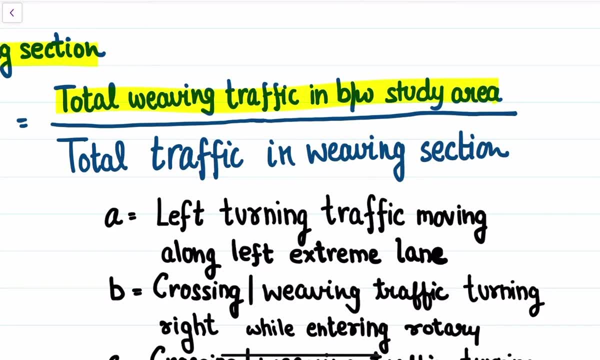 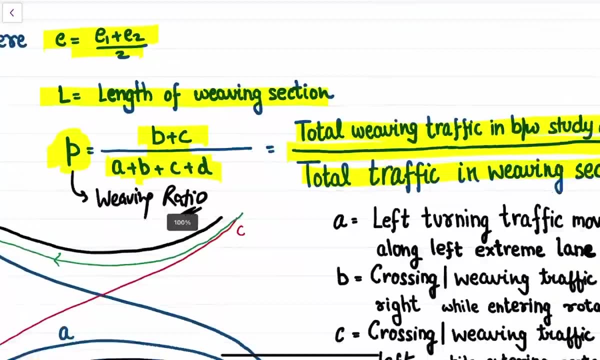 weaving ratio, which is the ratio of total weaving traffic in between the study area, total weaving traffic in between study area divided by total traffic in the weaving section, So which is equal to B plus C divided by A plus D, plus C plus D. Let us discuss this in detail. 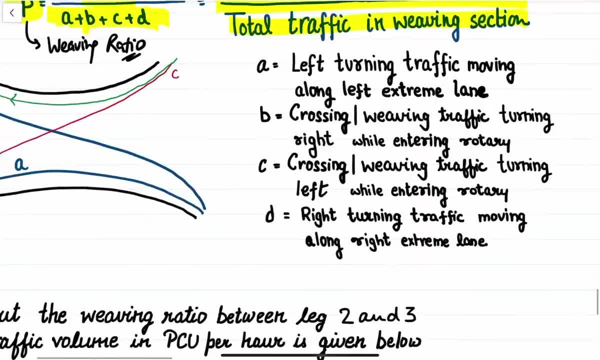 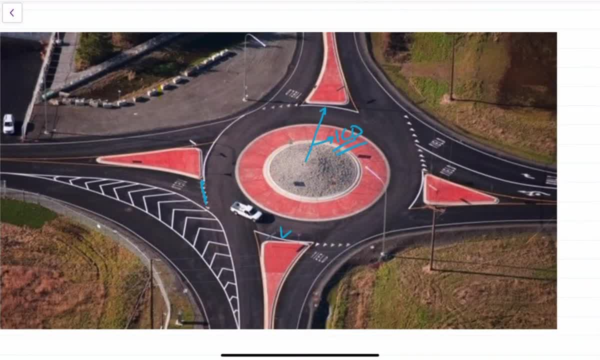 This is a very important term. So, basically, what happens is: what happens is that we have four legs of rotary. right, We have, let us say, four legs of rotary. We have leg 1, leg 2,, leg 3 and leg 4.. So what we do is, in order, in order to find out the weaving ratio, we assess 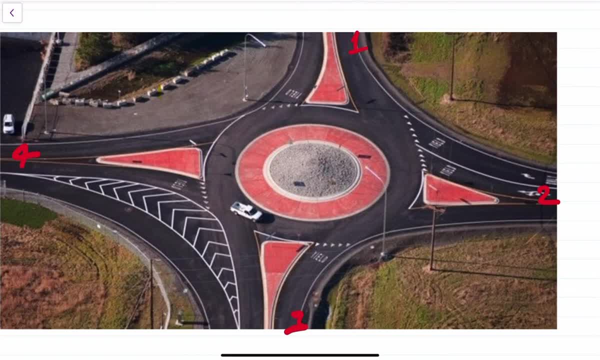 any two legs at a time And by considering the two legs at a time we try to find out the movement of the ratio between the movement of traffic in between the weaving section. So what we can do is time. either we can take traffic at 1 and 2 or we can take traffic in between 2 and 3. 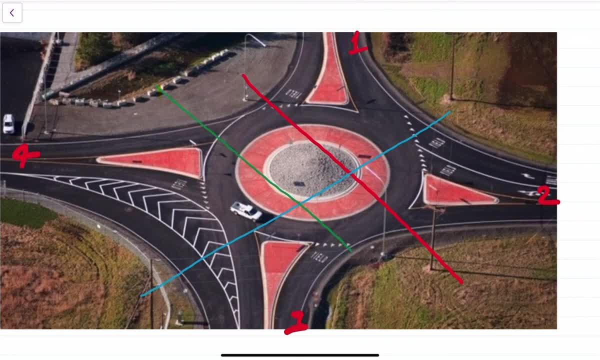 or we can take traffic in between 3 and 4- that is this section right- or we can take traffic in between 1 and 4. thing is, we are going. we are going to move in the clockwise direction. we are going to move in the clockwise direction, all right. so we consider at a time: 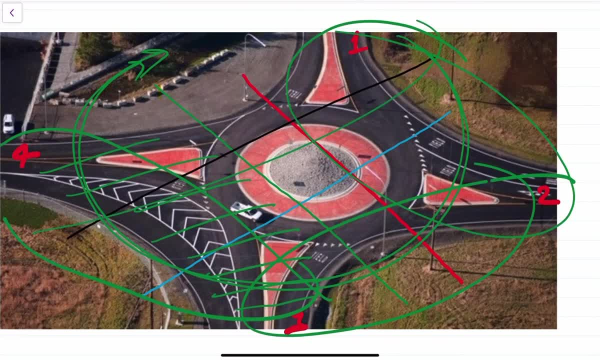 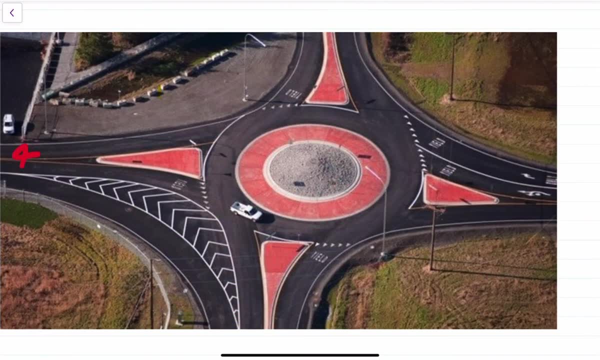 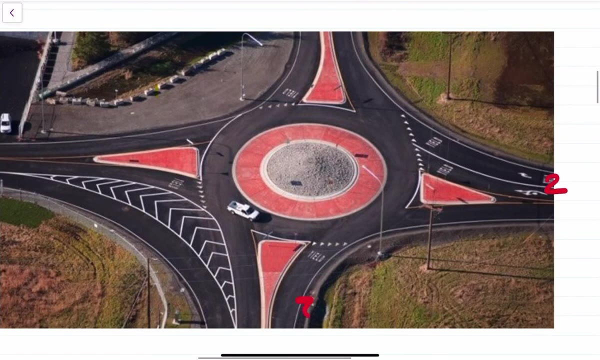 any two legs of the rotary and we try to find out the, we try to find out the traffic that is moving in between the weaving section. okay, so let us, for example, let us consider any legs. let us say we consider legs 2 and 3. right, we consider legs 2 and 3, so this section, that 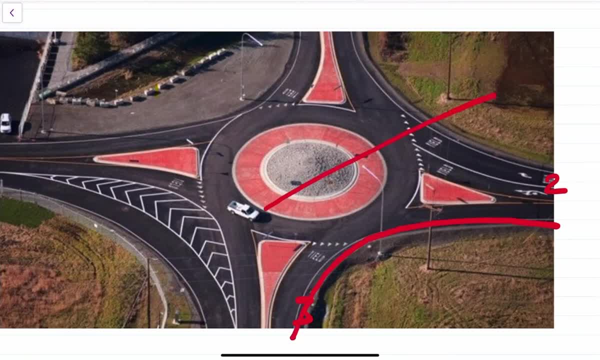 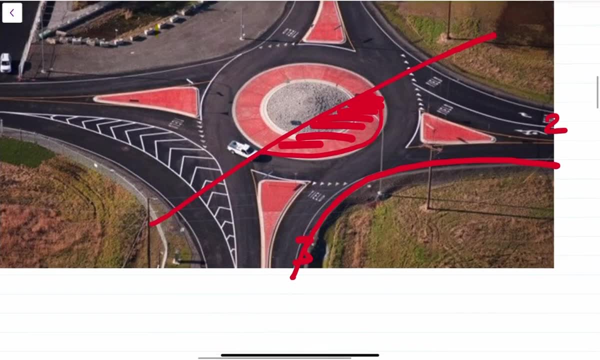 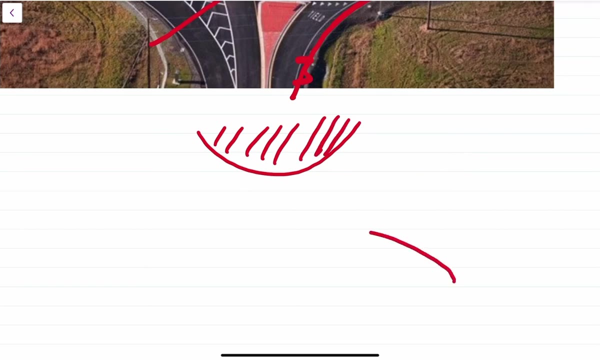 we are going to consider. is this section right, the section that we are going to consider? is this section right? So we will have this section. so let us represent it in the form of diagram. so we have a part of the central island and these are the legs right. these are the legs, let us say 2 and 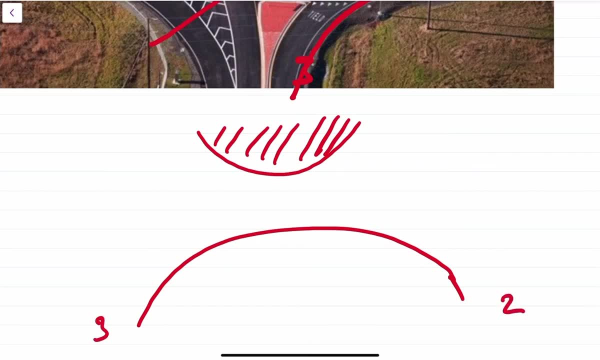 3, all right. so here what we try to find out. we try to find out the proportion of traffic moving in different direction. so, first of all, there will be a traffic that is coming from 2 and going to 3. there will be a traffic that will be connected to 2 and 3, right will. 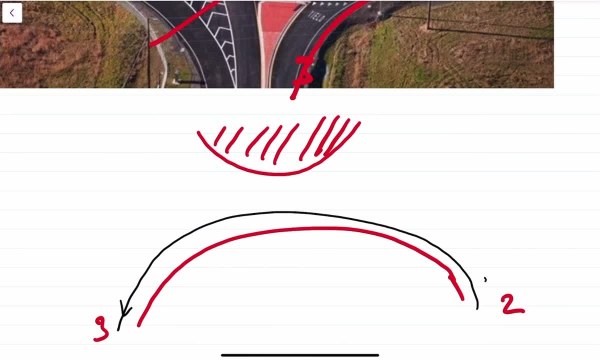 affect that direction, and so we will take the traffic that is moving from 2 and 3 and coming from 2 and going to 3, that is all the left turning traffic, so that we represent by A, that we represent by A. then we have a traffic that is moving, that is coming from. 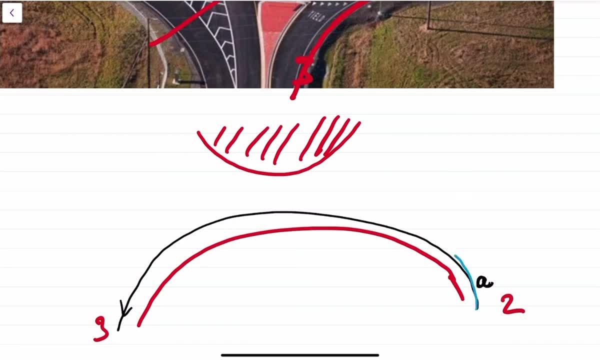 1 coming from 1 and may be going to some other leg. the leg may be leg 3 or leg 4. got it coming from leg 2 and going to some other leg. the leg may be leg number 4 or leg number 1, right. 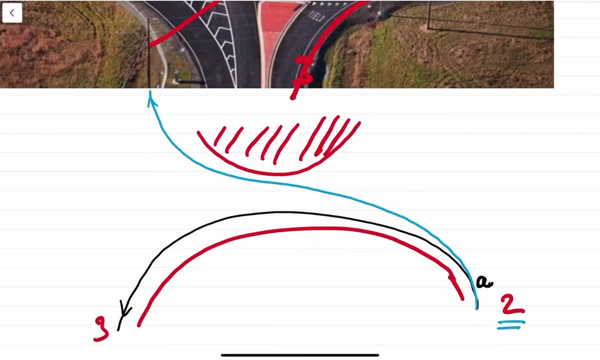 it can. so that is represented by B. that is represented by B. A is the left turning traffic coming from. the traffic is coming from 2 and going to 3. traffic coming from 2 and going to 3. that is what we call as the A when traffic is coming from 2.. 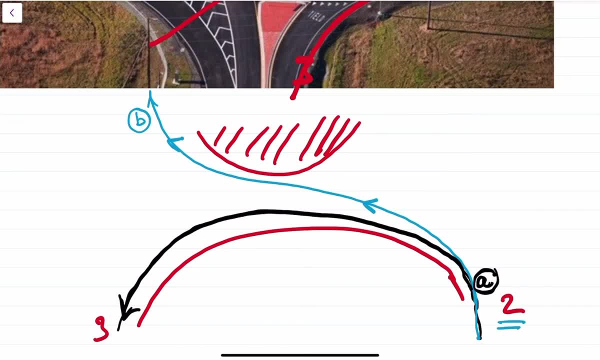 But going to some other leg apart from leg 3, that is, in this case leg 4 and 1 is called as our B. then there will be traffic from the other legs of the rotary that will be coming and going to leg number 3. in this case, the traffic can come from leg 4 or leg 1. so when 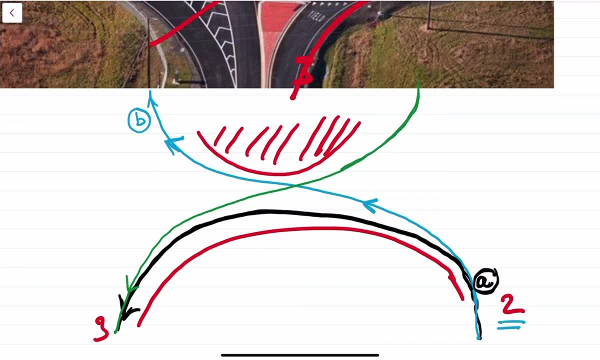 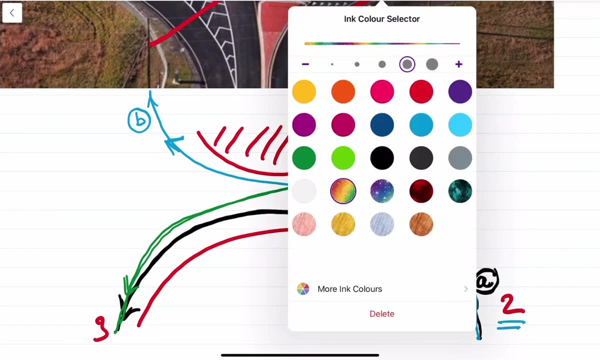 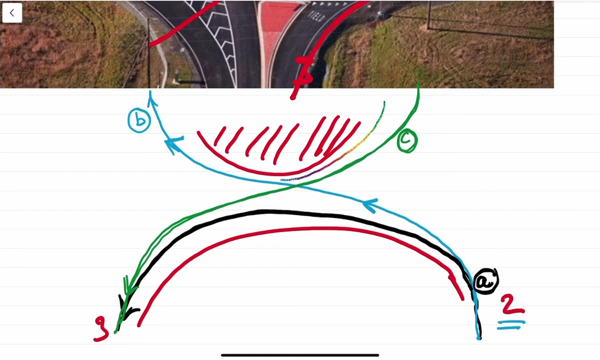 it comes from some other legs of the rotary and moves into the leg 3, that will be called as the C that we call as that, we call as C right, and then there will be a traffic. there will be a traffic that is neither coming from 2, neither going to 3, but is using this weaving. 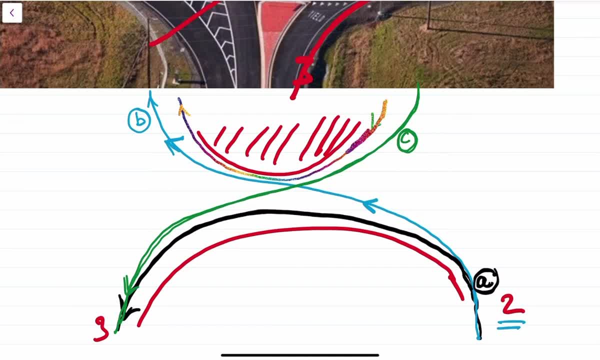 section right. it is using this weaving section. it is using this weaving section. that is using this weaving section To reach to the respective leg. so that is what we call as the D right. I will again repeat the traffic that is neither coming from 2 nor going to 3, but is coming from some other. 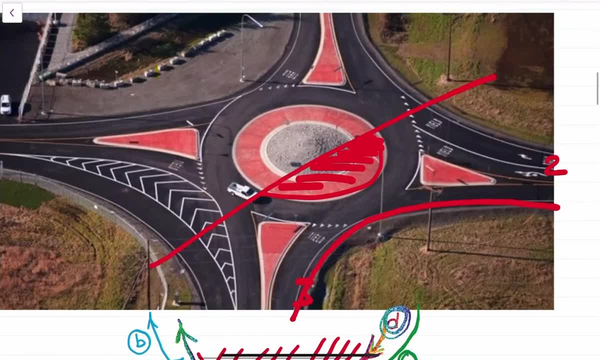 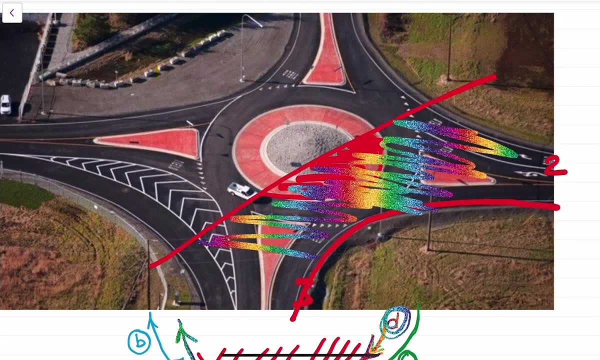 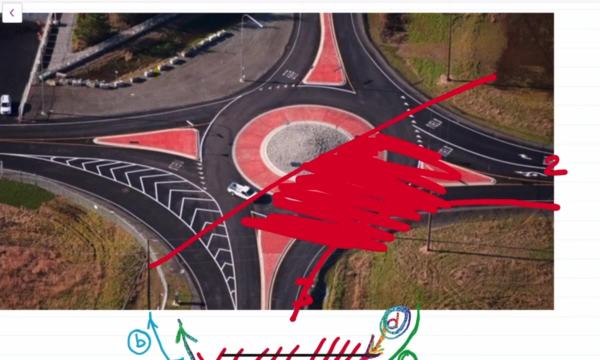 leg, but is using that weaving section, right? this is, this is our weaving section that we are, that we are considering. this is our weaving. this is our weaving section that we are considering. right, this is our weaving section that we are considering. so all the traffic that is. 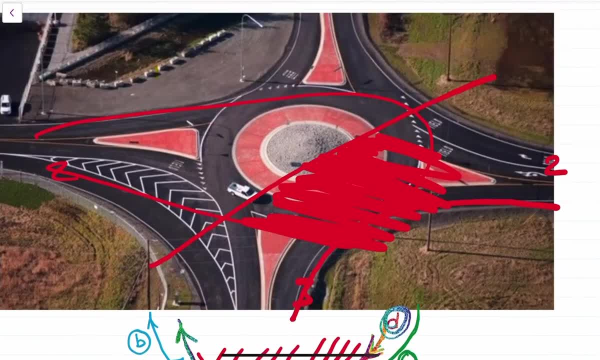 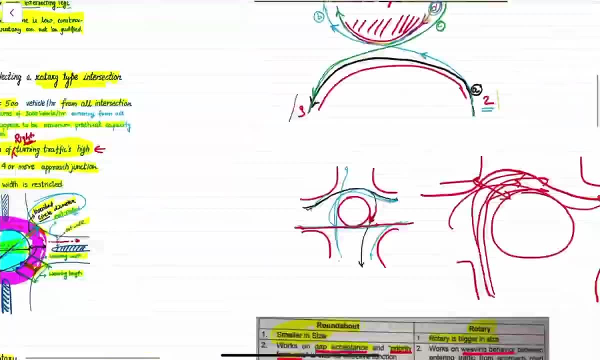 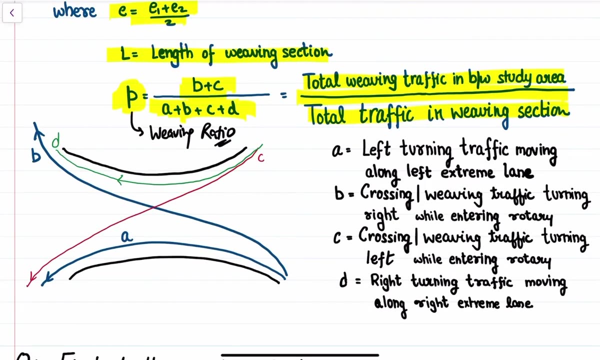 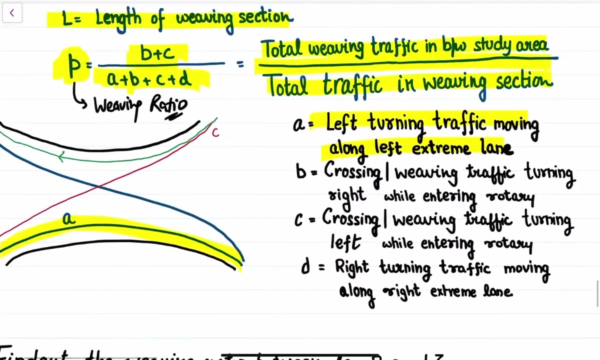 coming from this and using this weaving section, that is, that we will call as the D. I hope it is clear to you all. if not, then you can always ask in the comment section. So A is the, A is the left standing traffic moving along the extreme left lane, right or. 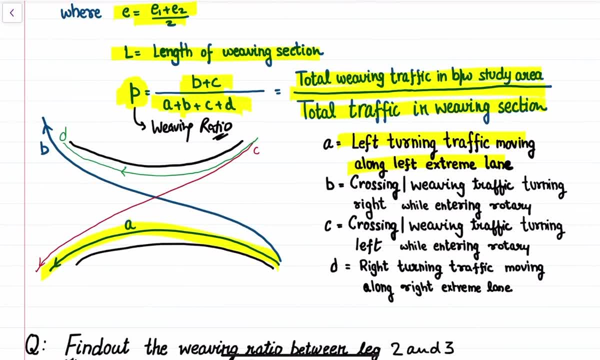 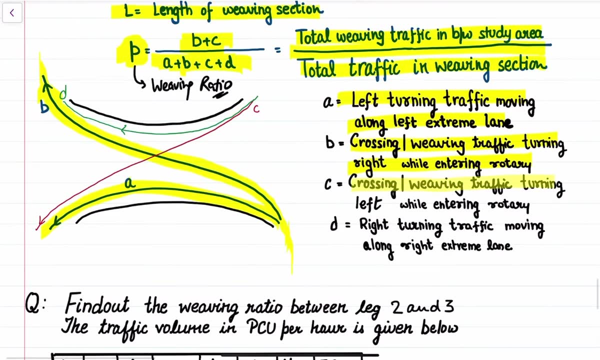 left corner, that is your A. B is the crossing weaving traffic turning right while entering the rotary crossing weaving traffic turning right while entering the rotary. so this means coming from the steady leg and going to some other leg. C is the crossing weaving traffic turning left while entering the rotary. so all the 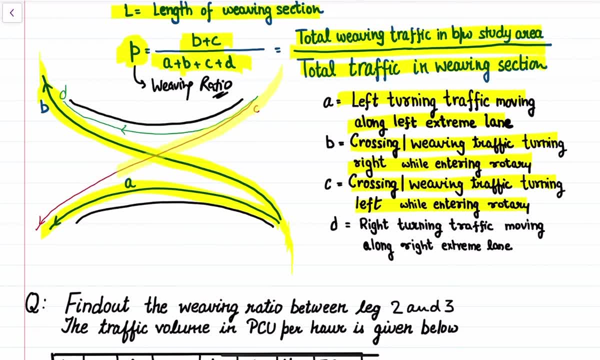 traffic that is coming from a different leg and going to the steady leg, and D is the right turning traffic moving along the right extreme lane. that is the left variable that we are considering here. we bless right. Thank you for watching this video. if you have any question, please do not hesitate to. 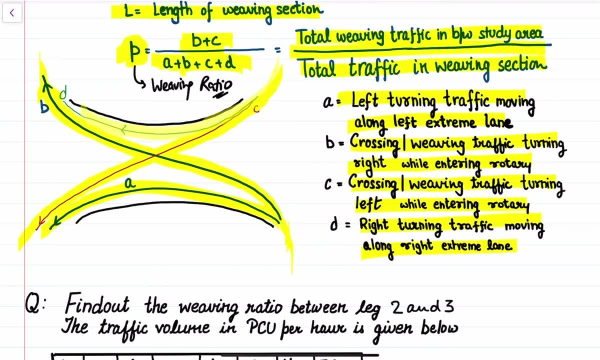 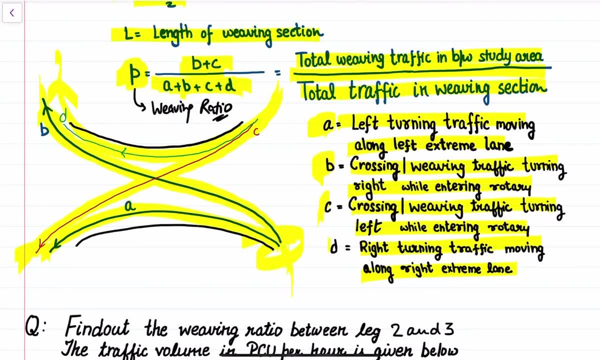 ask- and there will beер questions again and again as we come to the next part- is coming from any other lane and going to any other lane except our study lane? So that is what we define as the A, B, C, D. So your weaving ratio, your weaving ratio, 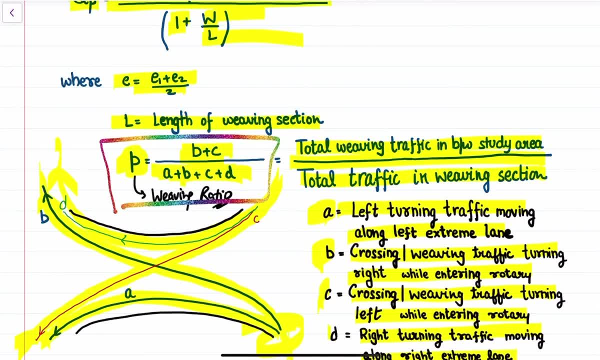 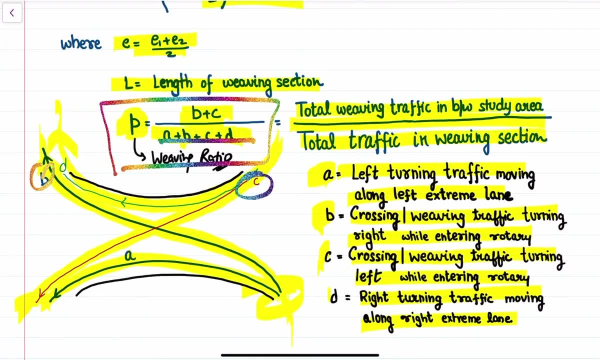 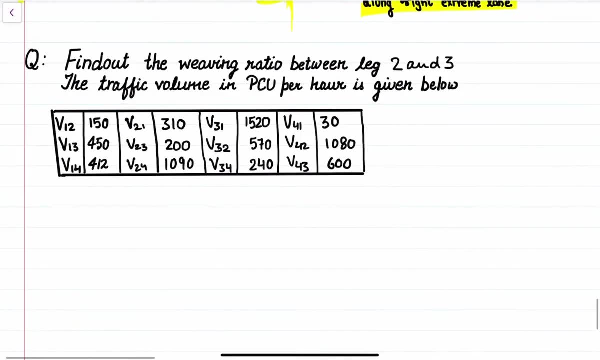 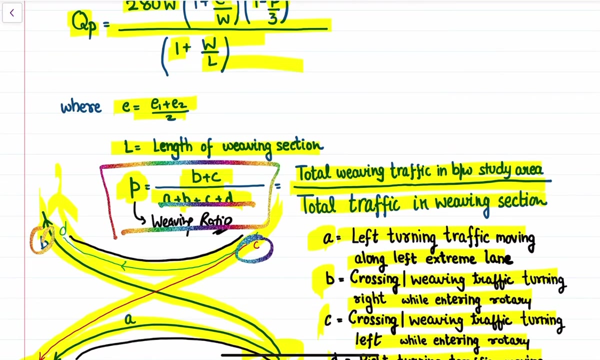 will be B plus C, B plus C divided by A plus B plus C plus D. that will be your weaving ratio. I hope it is clear to you all. If not, you can always ask. So let us just quickly do a quick numerical on this weaving ratio Rest, I think we will have a new video lecture. 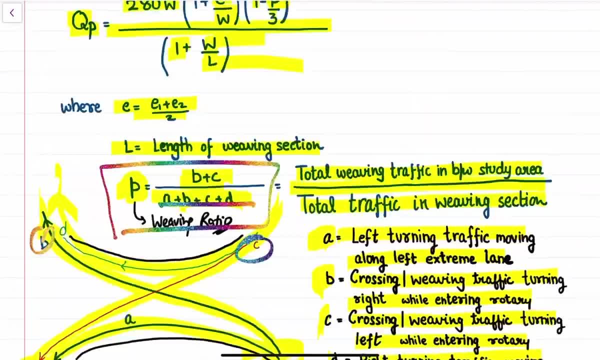 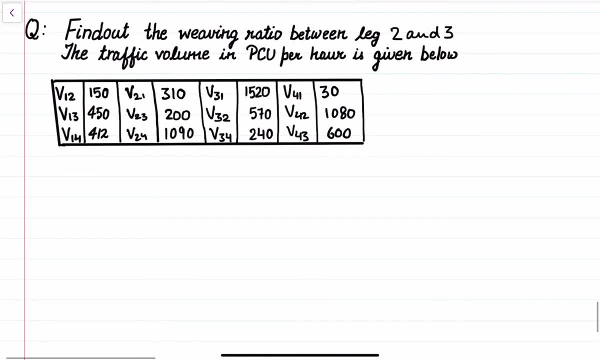 on that, but we will just discuss about this numerical on the weaving ratio. So the question is that we have to find out the weaving ratio between leg 2 and 3, the traffic volume in PCU RL. So what are the weaving ratios given in this table? So what we have is, first of all, let 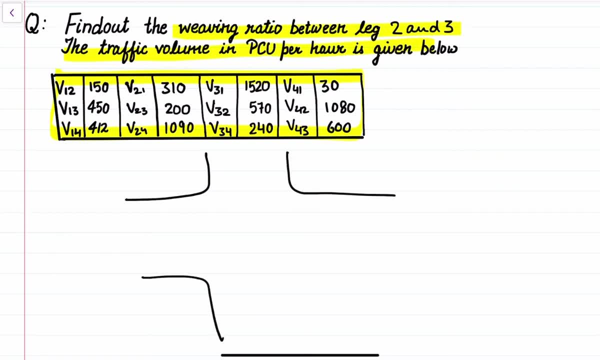 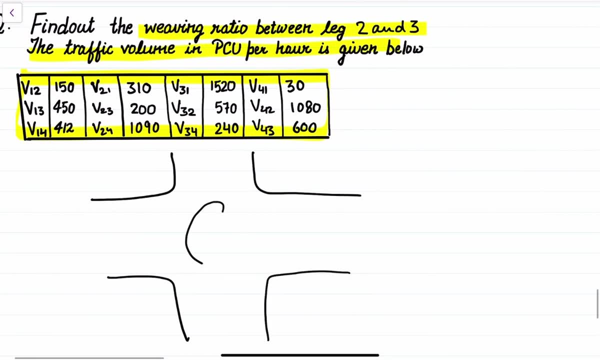 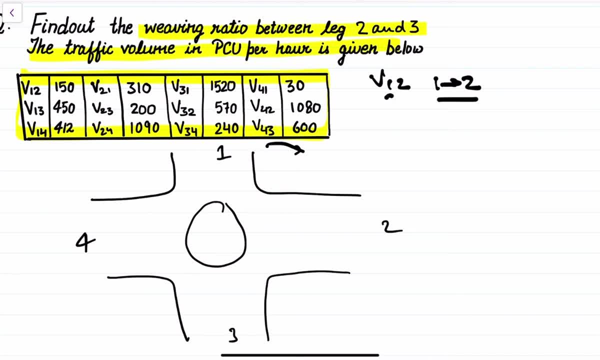 2, 1, 2, 1, 2, 3, 1, 2, 2, 1, 2, 1, 2, 1, 2,. everything means first means coming, second means going. So we have to find out between leg 2 and 3.. Let me just 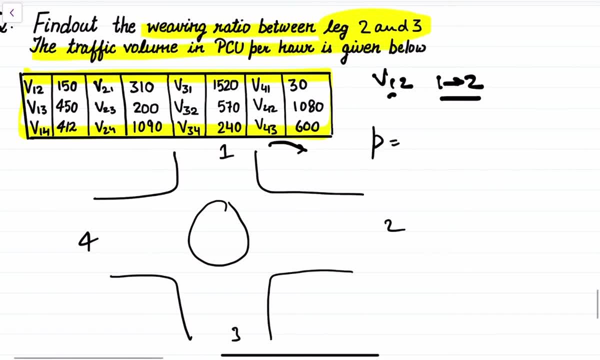 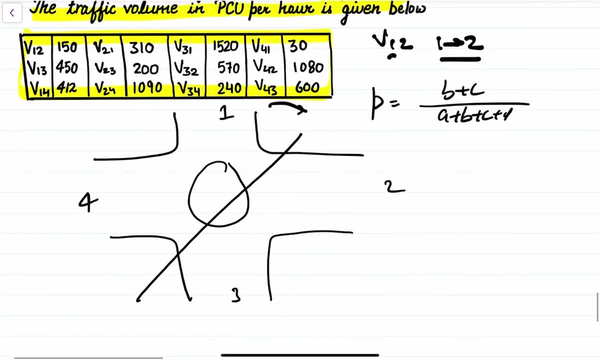 quickly write down the formula: Weaving ratio is B plus C, divided by A plus B plus C plus D. So we have to find out between 2 and 3.. This is 2 and 3.. Right, So let us draw the. 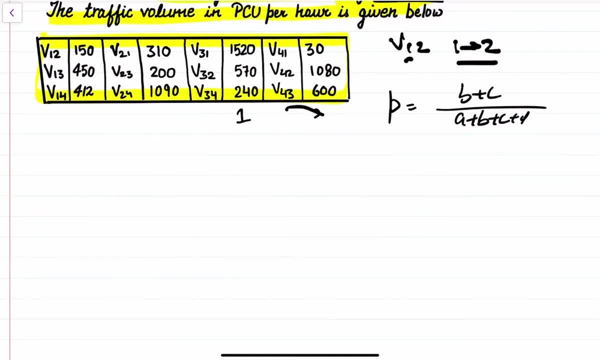 diagram for 2 and 3.. Quickly, let us draw the diagram for 2 and 3.. So we have leg leg 3 and leg 4.. All right, So we have to do the diagram with web3.Now it looks like. 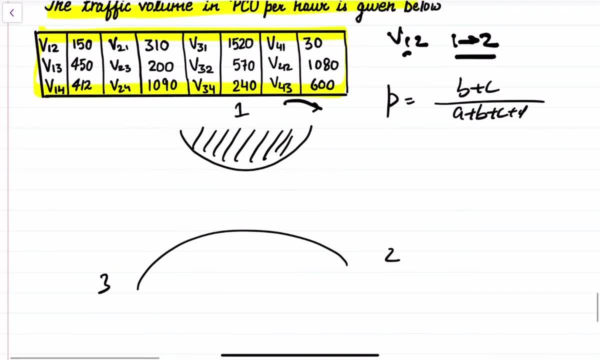 finally, we have wide equivalence. Okay, So exactly. So. the diagram should be exactly So. this is the diagram and this is the corresponding in the expression. This is the in between. This is the in between is leg 2, this is leg 3.. So first of all, we have to find out: A. what is A Vehicle coming from? 2. 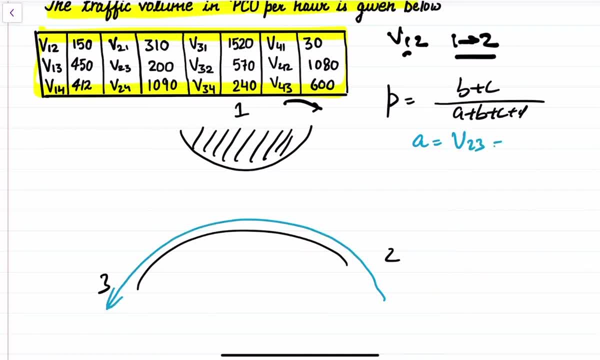 going to 3.. A will be V23.. V23 value is 200.. V23 value is 200.. B coming from 2 and going to some other leg Here. in this case, other leg may be 2 to 3 or 2 to 4.. So sorry, 2 to 4 or 2 to 1.. So. 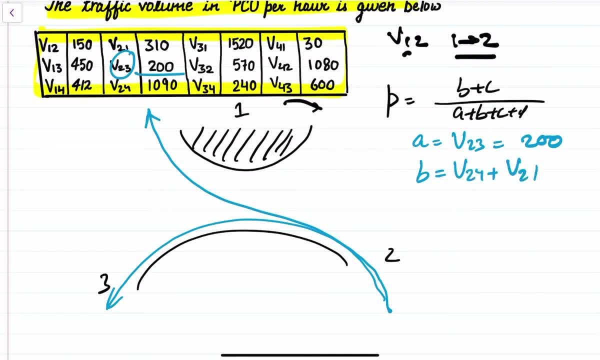 we have 2 to 4 plus V2 to 1.. So V24 is 1090.. V21 is 310.. So the value is 1400.. Just keep checking if I am doing any calculation mistake. C- C is all the vehicles coming from the other. 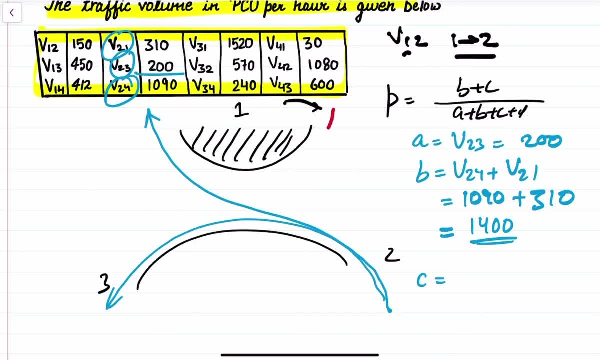 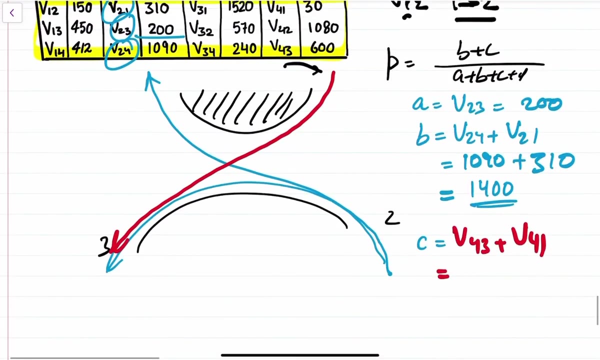 legs and going to 3.. In this case, the other leg will be V23.. Either it can be 4 or it can be 1.. It can be 4 or it can be 1.. So we have vehicle coming from 4 going to 3.. Vehicle coming from 4 going to 1.. Sorry, sorry, Vehicle coming from 4. 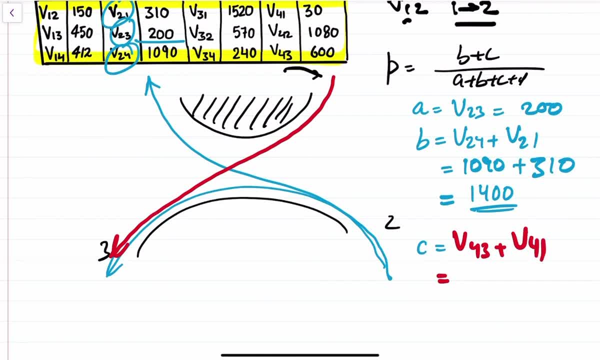 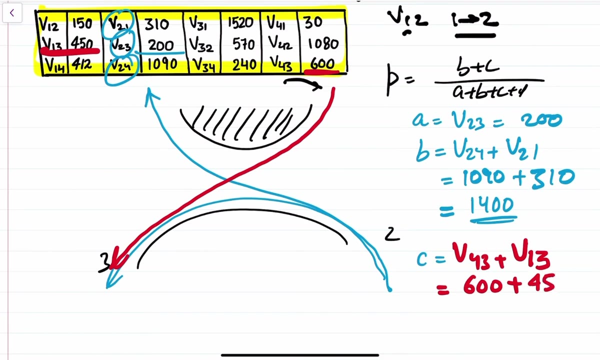 going to 3 and vehicle coming from 1 going to 3.. Vehicle coming from 1 and going to 3.. Right, So V43.. V43 is 600. And V13. V13 is 450.. V13 is 450. So this will be 1050.. Talking. 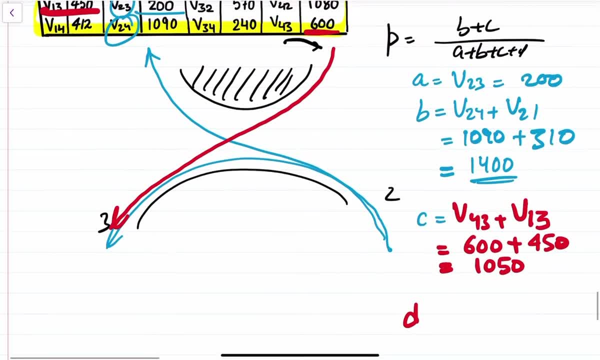 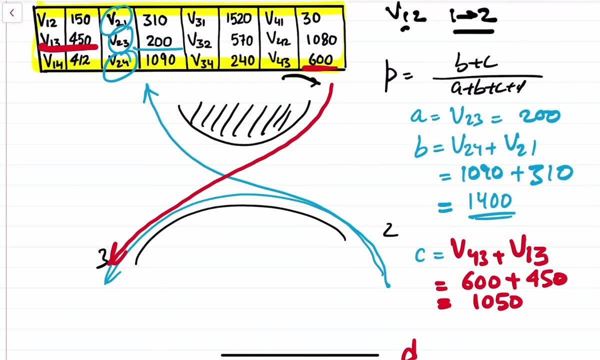 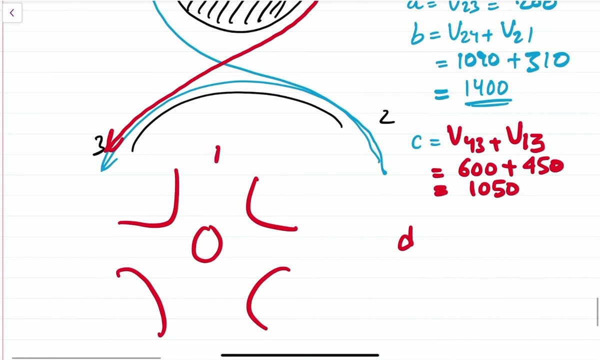 about D. D is any vehicle that is coming from some other leg and going to some other leg. So in this case Either a vehicle Right. either a vehicle can come from 1 or can come from. either can come from 1 and go to 4 or 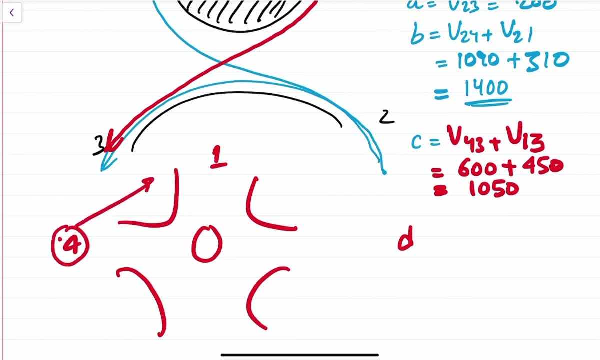 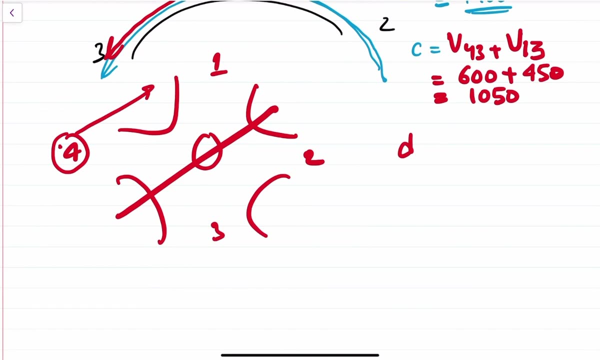 is coming from 4 and going to 1.. So, which we are going to take? We are going to take the vehicle that is using this weaving section. This is 2,, this is 3, the vehicle that is going to use this weaving section. So, if you see here, if you see here a vehicle coming, 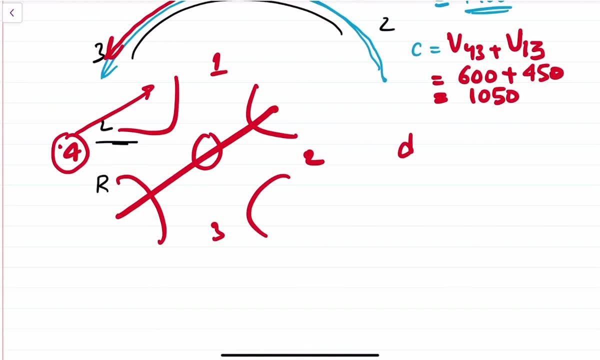 from 4, this is left. this is right. we simply turn left. right Vehicle coming from 4 will simply turn left and go to 1.. It will not use this weaving section, While if a vehicle coming from 1 has to go to 4, he has to go through this weaving section and then go to. 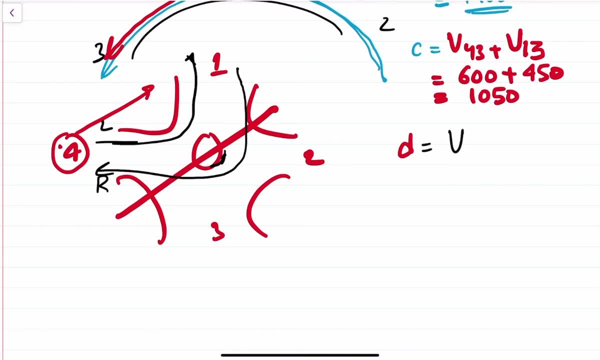 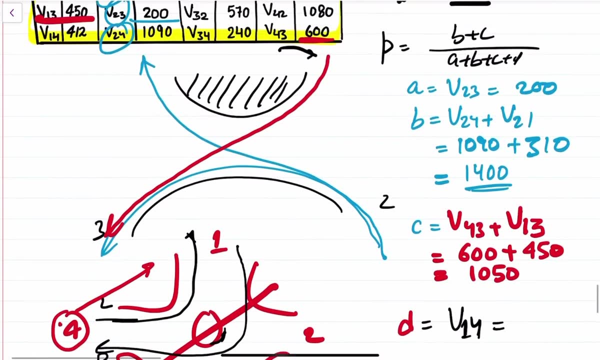 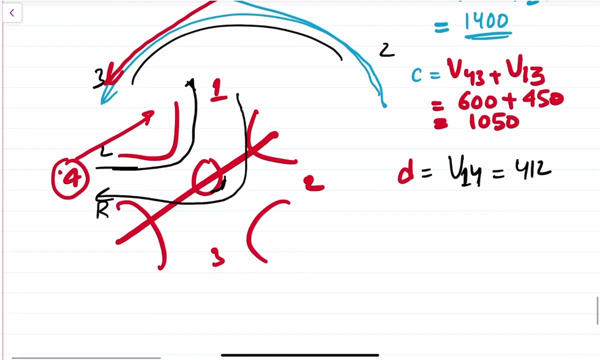 left 4.. So D in this case will be V14, right, D in this case will be V14, right, And the value of V14 is V14 is 412.. This will be 412.. Clear, So just put the value: C will be D plus C. So 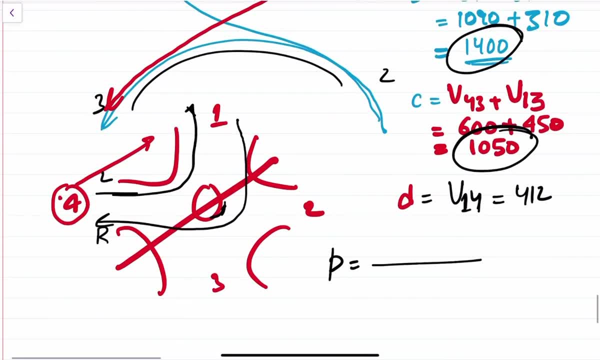 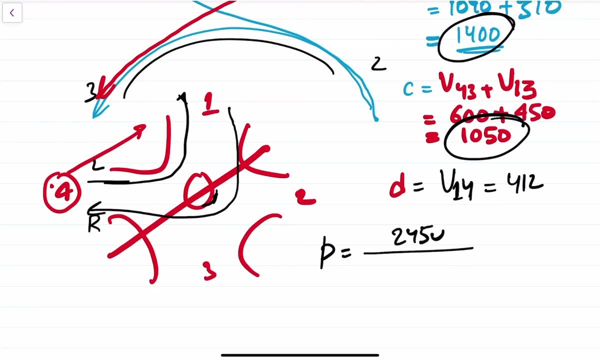 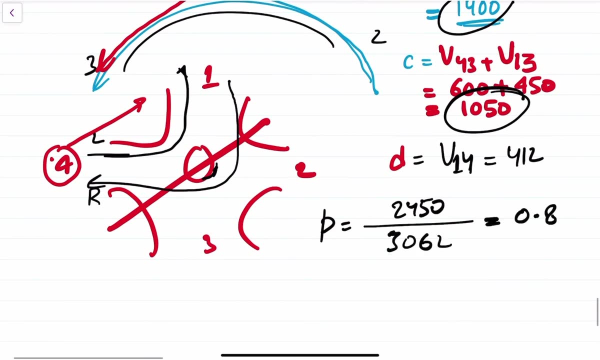 D plus C. this will be so. this will be 2450 divided by A plus D plus C plus D. right, That will be 3062.. So the value will be 0.80.. Okay, The value will be 0.80.. Okay, So the weaving ratio is 0.80.. Okay, So you can try. 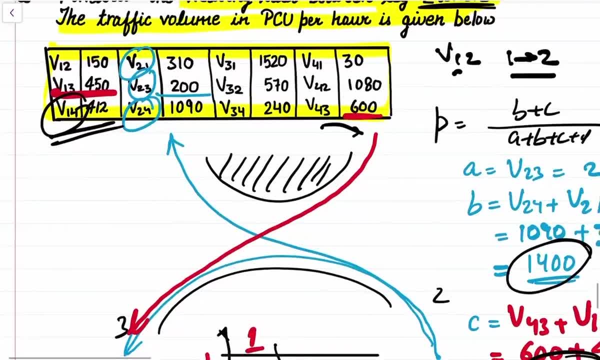 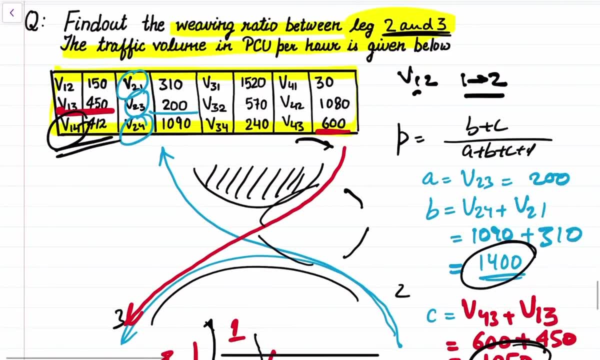 among by yourself. also, you can try to find out for like 1 to 2,, 2 to 3,, 3 to 4 and 4 to 1, right, You can find out the weaving ratio and just you can post the values in. 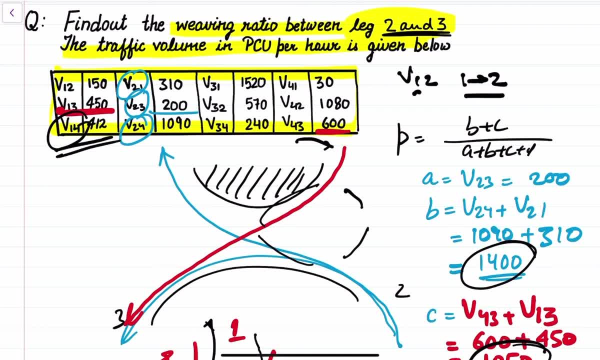 the comment section and we will see who post the right values right. And if, in case you have any doubt, we are going to do some more miracles in the coming lectures, So keep a track of the upcoming lectures. Okay, So I hope this video was useful to you Everything. 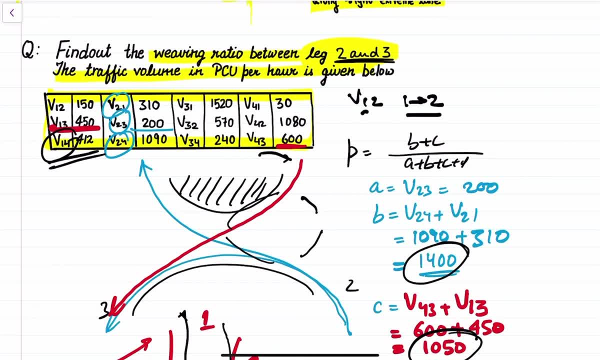 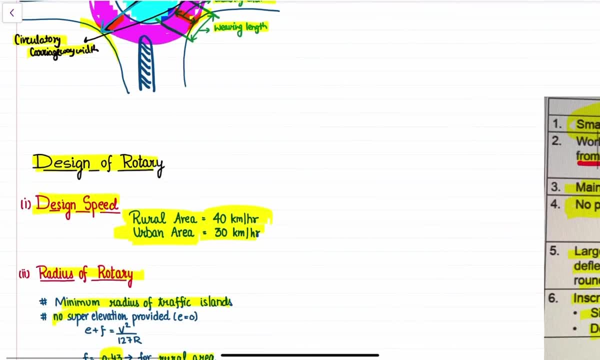 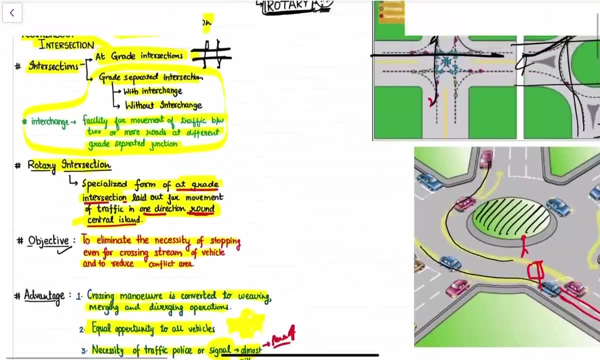 the theoretical concept of rotary in roundabout and stylized intersection is clear to you, right? If this video was useful to you, make sure you like the video. Share this video with your friends and do subscribe to the channel. Your subscribing motivates us to. 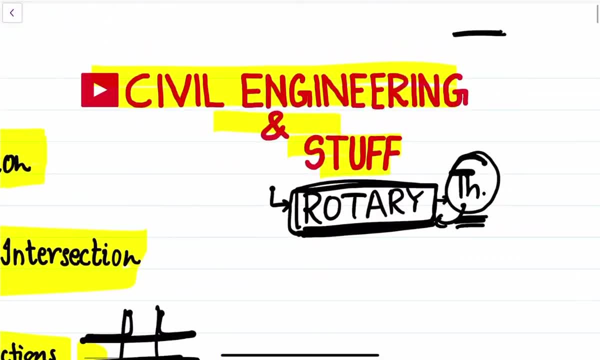 make more videos like this. If you have any suggestions, do post in the comment section. So thank you for watching. Have a nice day.